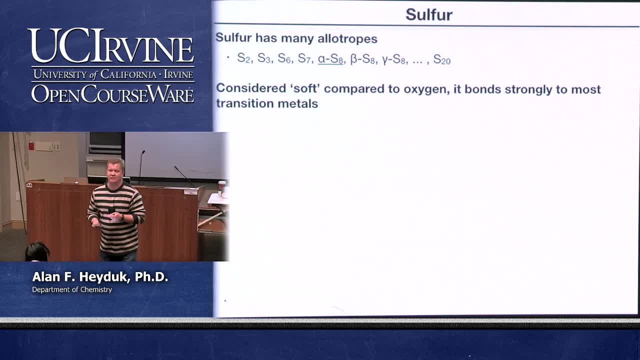 You probably were already introduced to S8 because it's one of everybody's favorite symmetry questions, and so on and so forth up to S20.. S8 is by far the most common elemental form of silicon. Of course, sulfur. wow, we're going to have one of those days where I can't keep track. 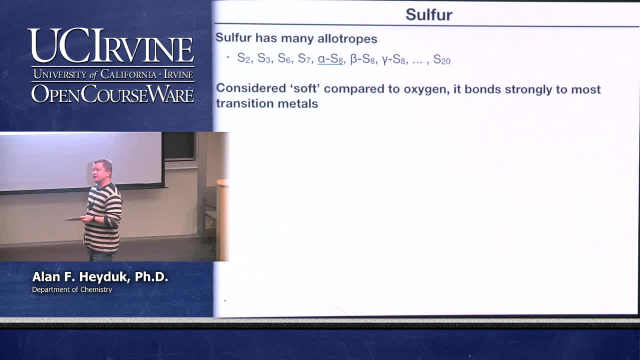 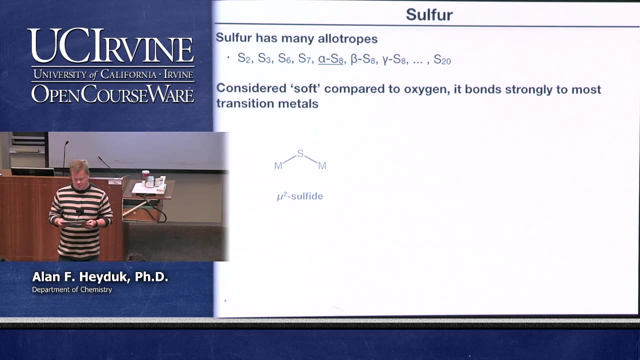 of what I'm saying. So obviously, because we're dropping down from a 2p element of oxygen to a 3p element of sulfur. sulfur is considered to be soft compared to oxygen. It's a very, very good donor atom towards transition metals. 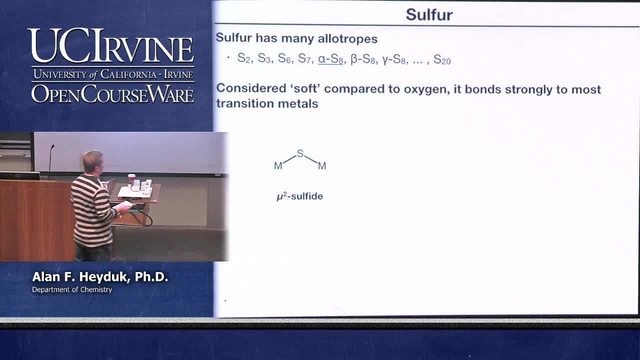 So we'll see a lot of sulfur-type ligands for transition metals, and then the other thing that sulfur by itself does really well is form bridging species okay, and so a lot of times you'll have 2p, So you can have two transition metals with a single bridging sulfur. 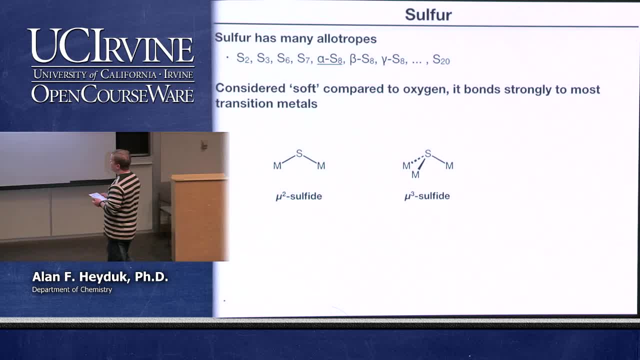 We would call that a Mu2 sulfide. You can have Mu3 sulfides, So this actually looks like the sulfur is capping a trigonal face that's presented by three different transition metals, And you can also have a Mu4 sulfide. 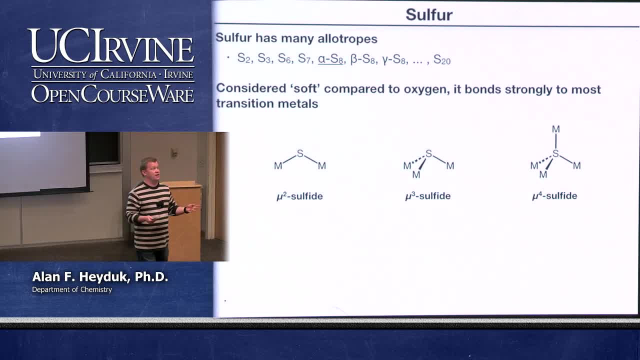 So now this is kind of weird, right, because it looks like sulfur is making too many bonds. right? We know oxygen can only make really two bonds. Sulfur, in this case, can make four bonds to different transition metals, and we'll talk. 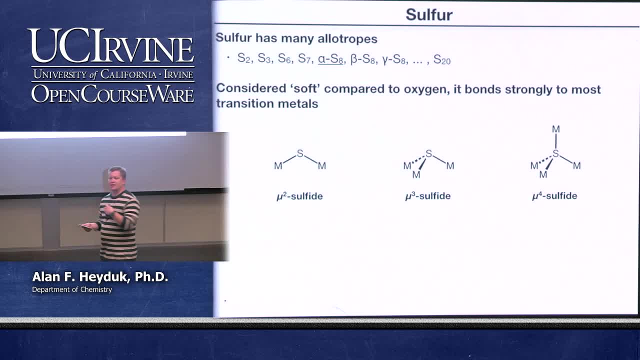 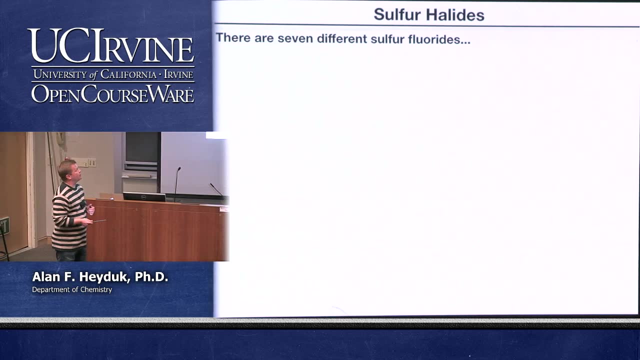 exactly about how that happens, but in a way it's kind of satisfying because you can obviously see that the sulfur can adopt basically sp3 hybridization, right Okay, So when you're talking about sulfur compounds, you have to talk about the halogen complexes. 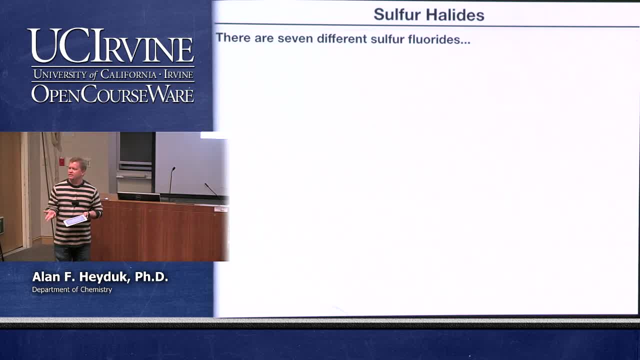 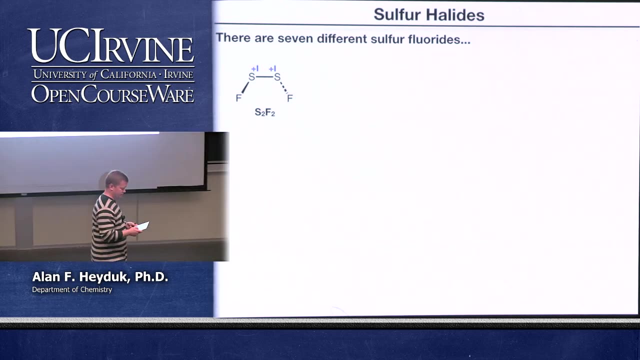 of sulfur. And again, we don't really think about this very often, right, Because we typically think of p-block elements bonding to metals or something like that, not to other p-block elements. But it turns out you can make S2F2, probably not a surprise. 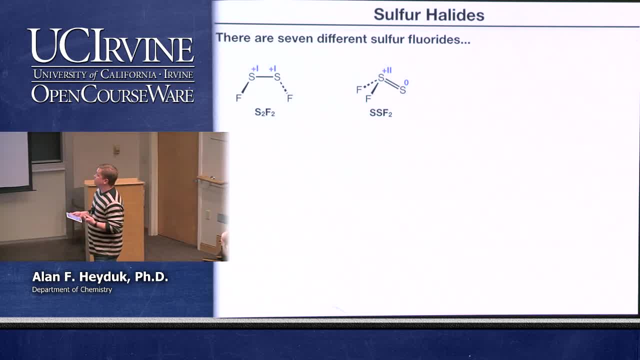 In that case the oxidation state of both sulfurs are plus one because, I'll remind you, with oxidation state we assign both electrons in the bond to the more electronegative atom. So in the case of something like sulfur hex, The S2F2 complex, the electrons in the sulfur fluorine bond go to the fluoride, because it's. 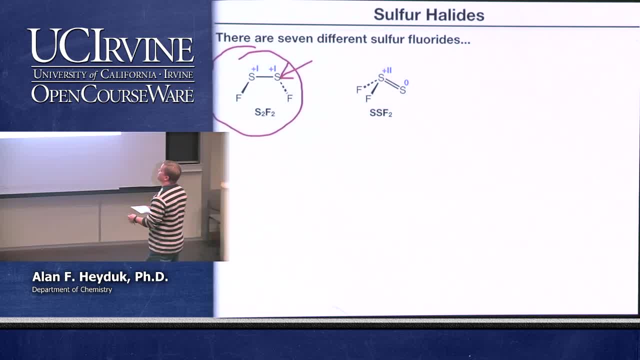 more electronegative. The electrons in the sulfur-sulfur bond get split evenly when you're assigning the oxidation state. This again differs from formal charge. If we were assigning formal charges, every single bond would get split evenly. Another interesting one: S2F2.. 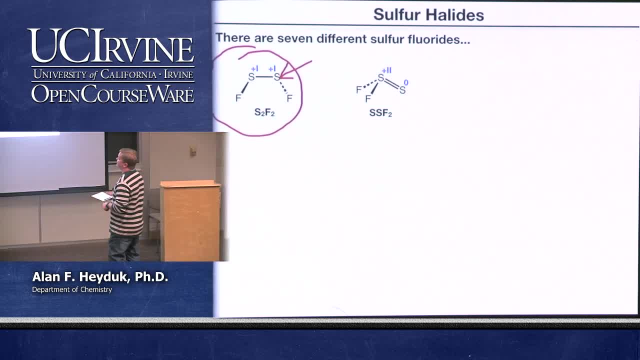 You can see I've written it out as S-S-F2 to indicate that the sulfurs are different. Obviously, one sulfur has two fluorines bonded to it. The other has the sulfur-sulfur double bond. So in a weird kind of way I look at that and I think it kind of looks like a ketone. 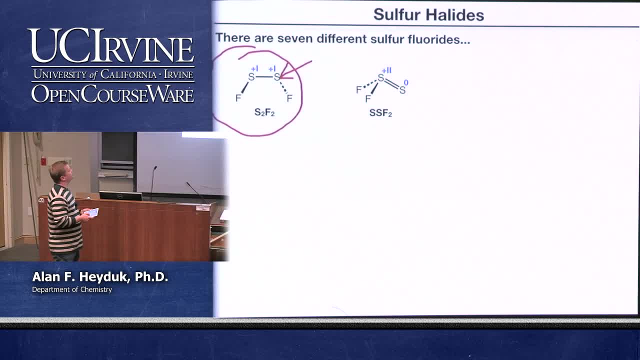 In a weird way. I'll admit it's not a perfect comparison, but you get what I mean. You can have S-F2, again, probably not surprising. It kind of looks like a ketone. It looks like water. We can get more complicated. 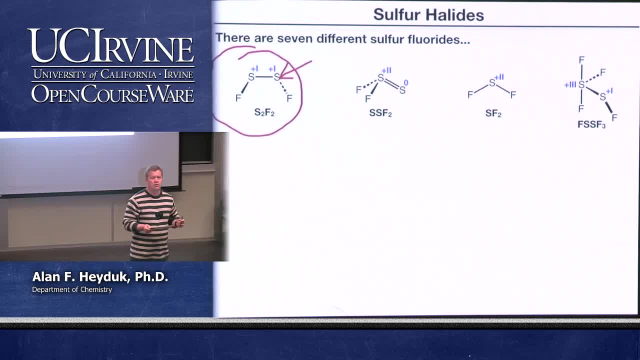 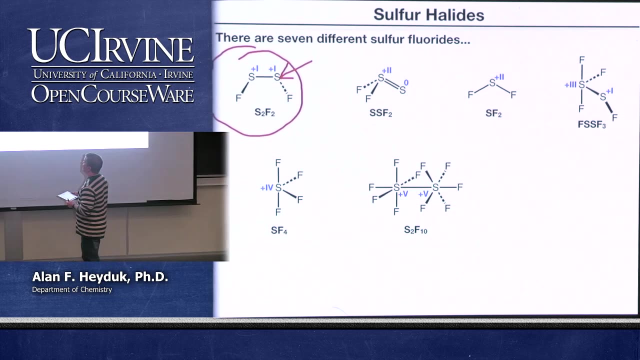 That one looks really weird. So we have a sulfur-sulfur bond. One of the sulfurs is bonded to a single fluorine. The other sulfur is bonded to three fluorines: S-F4, S2F10.. Okay, So we can add lots of fluorine. 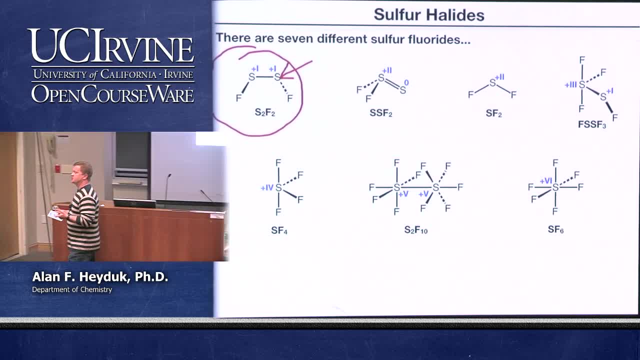 Fluorine to sulfur, And I think one of the things that this drives home is that fluorine, which we'll talk about in a minute or two, is a very, very, very oxidizing element. Right Again, if we're assigning oxidation states, the sulfur in that S-F6 molecule is in the 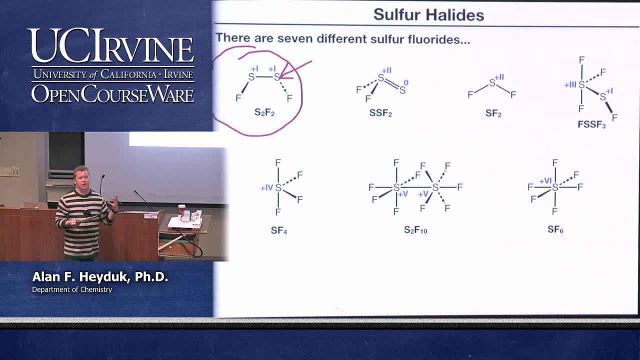 plus six oxidation state. If we think about where sulfur is on the periodic table, we always talk about those elements being the most electronegative. there are Right, Fluorine is first, Oxygen is second, Chlorine is third, And then it kind of starts to spread out. 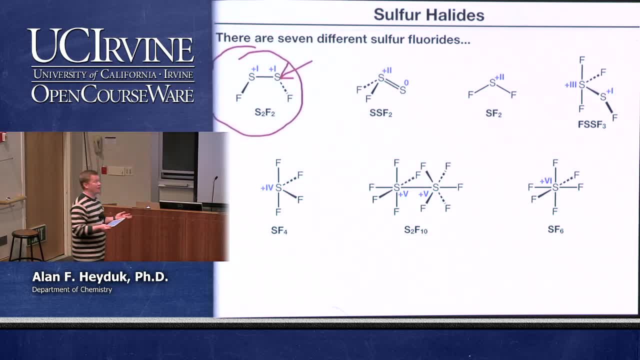 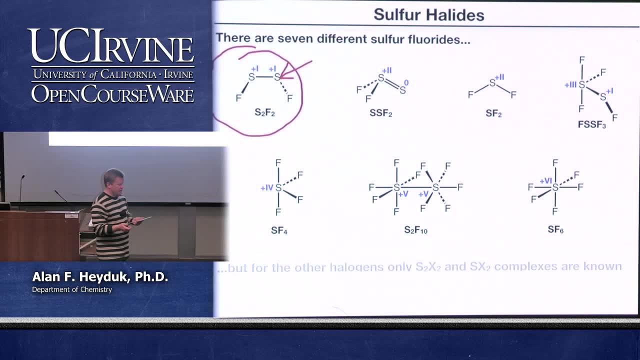 But largely we think of sulfur as being a relatively electronegative element, yet we're still taking it all the way up to the plus six oxidation state with fluorine. Now again, the ability of fluorine to act as an oxidizing agent is highlighted by the. 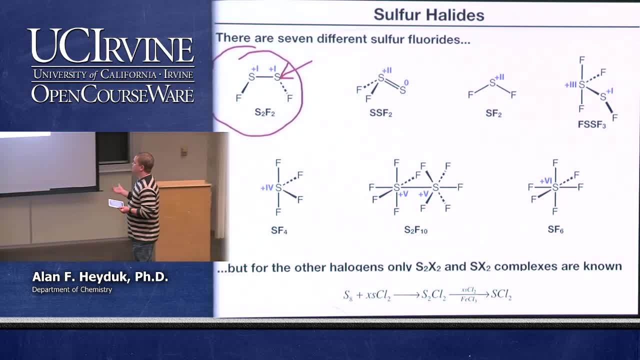 fact that if you use a different halogen, you're not going to reach those fantastically high oxidations. You're going to reach those fantastically high oxidation states for sulfur. So S8 will react with chlorine to make the analog to this compound in the top left, S2Cl2.. 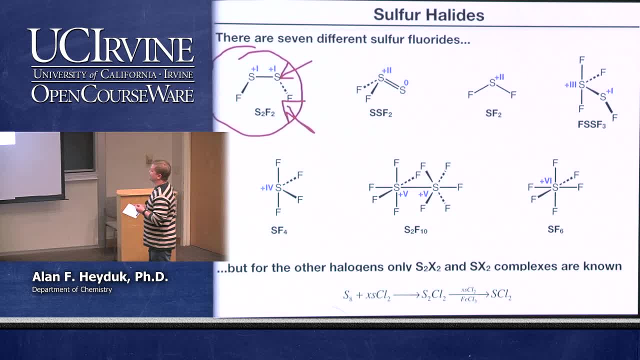 And if you have excess chlorine in an iron-lewis acid catalyst you can get to the chlorine analog of Sf2.. But that's it. You don't make any of these other oddball structures or ultra-high oxidation states of sulfur, And of course the same is true for bromine or iodine. 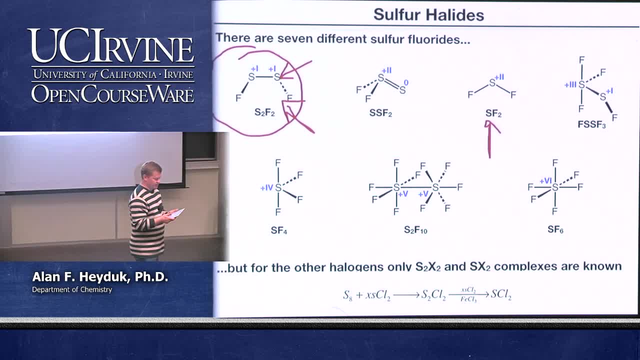 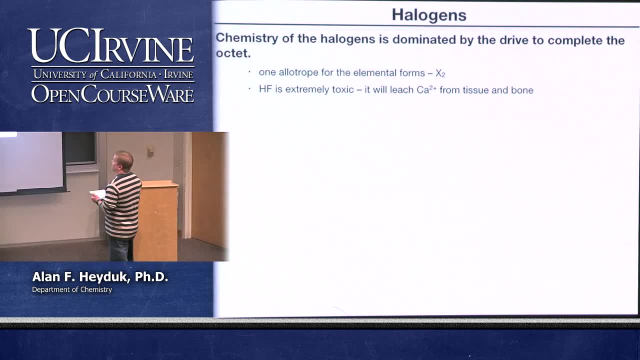 They don't have the oxidizing agent, They don't have the oxidizing power to generate, for instance, Si6. Just doesn't happen. So, speaking of the halogens, the halogens are a case where the octet rule works pretty. 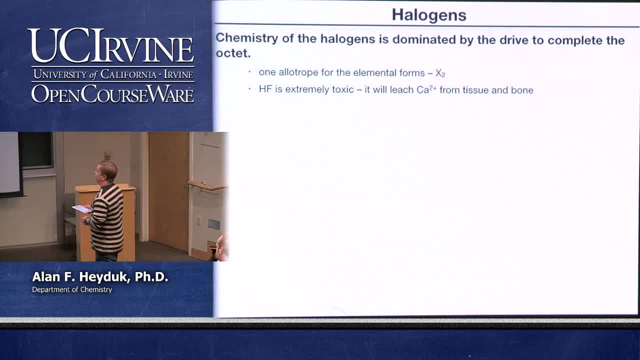 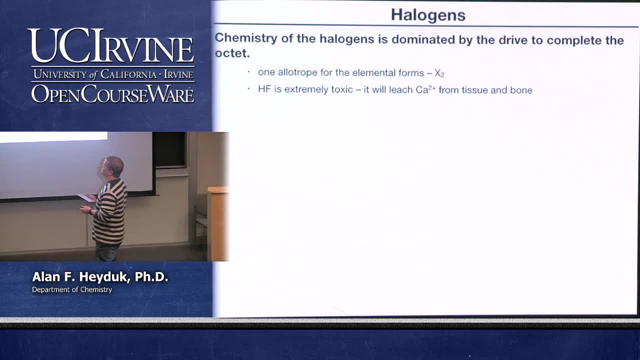 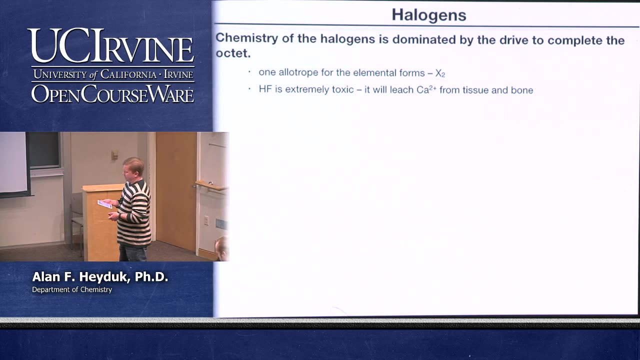 darn well. Halogens like to complete their octet. Basically, all they need to do is take up one electron. So for all of the elements, the only allotrope is the X2.. So fluorine gas, Fluorine gas, bromine liquid, iodine, solid HF- bad news. 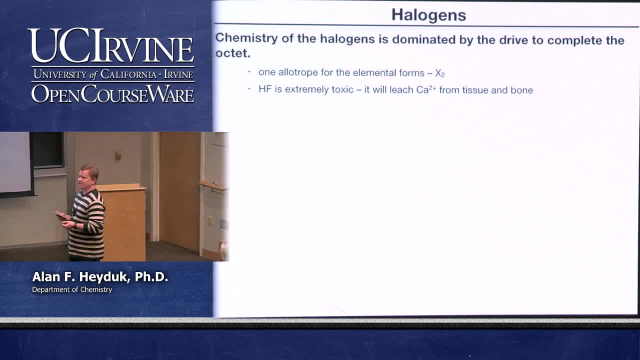 You don't want to get exposed to HF. It will leach calcium from your bones. Fluoride is so calcium-ophilic it will literally take the calcium from your bones. Worse, it'll take calcium from your ion channels and kind of like: well, it's over, right. 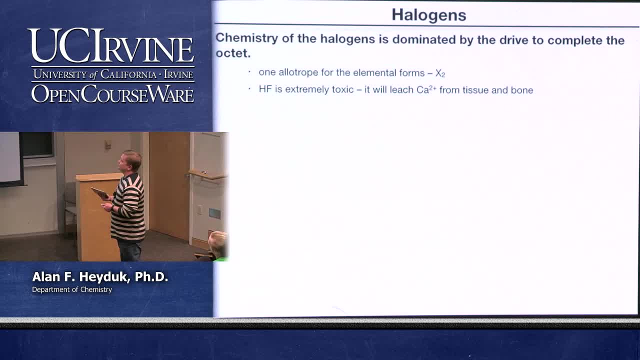 Calcium is used in communication, So it's really kind of neat. Well, no, it's not. If you get a drop of HF on you, it will literally burn right through your skin, right through your flesh, right till you get to the bone. 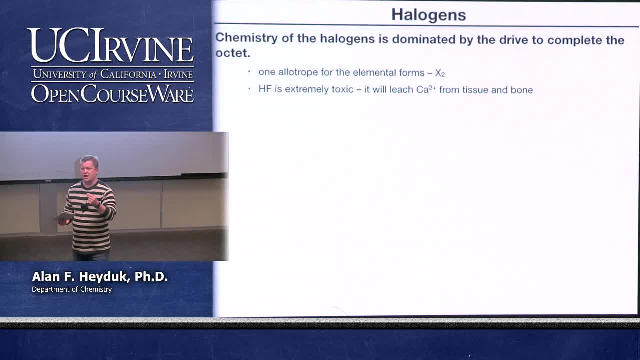 You have to treat it with basically a toothpaste-type material that has a bunch of calcium in it that tries to bind up the fluoride before it finds fluoride from your body. Pretty darn, let's see. okay, this is being problematic, okay. 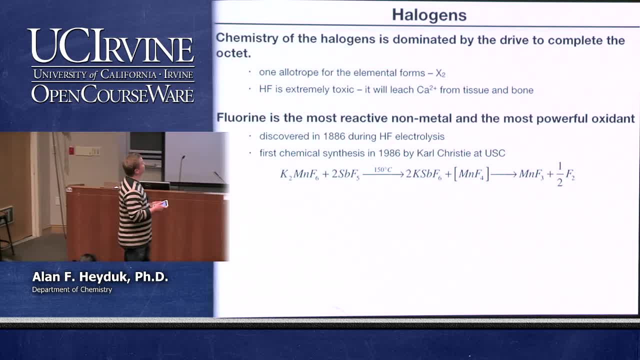 So anyways, Bottom line, Try not to get exposed to HF. Okay, So fluorine- we just mentioned incredibly powerful oxidizing agent. It's the one element that will allow many other elements on the periodic table to reach their terminal oxidation state, like we just saw for sulfur. It was discovered a long time ago from the electrolysis of HF. so we talked about electrolysis experiments. You take an HF solution, You basically pass a current through it. Hydrogen bubbles off of one electrode and fluorine gas bubbles off the other. 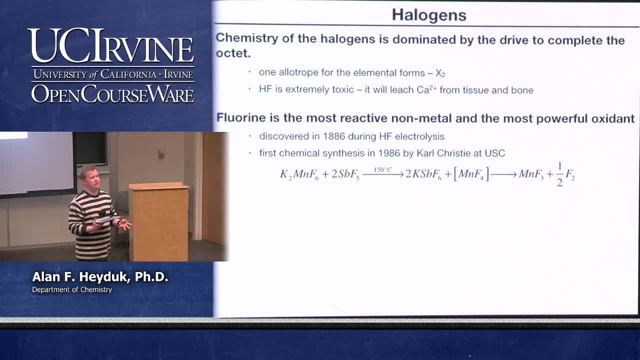 But the first chemical synthesis, ie non-electrochemical synthesis, that's not a typo- 1986. Of course you guys were you guys born in 86?? Oh geez, I have bad news. You just all lost 20% on your grade in the class. 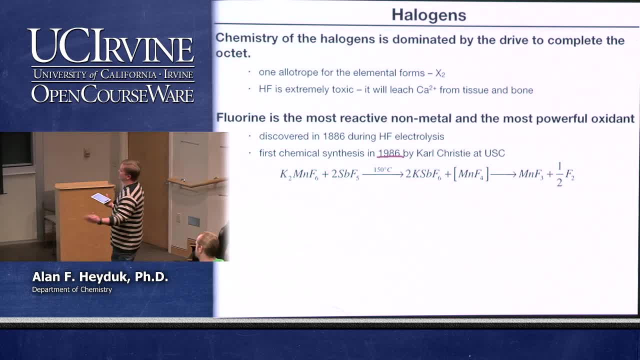 I was in high school in 1986, thanks, That wasn't funny. So 1986 seems like just yesterday to me. You don't remember it, but that's the first time fluorine gas was synthesized in the lab. To me that just seems crazy, right. 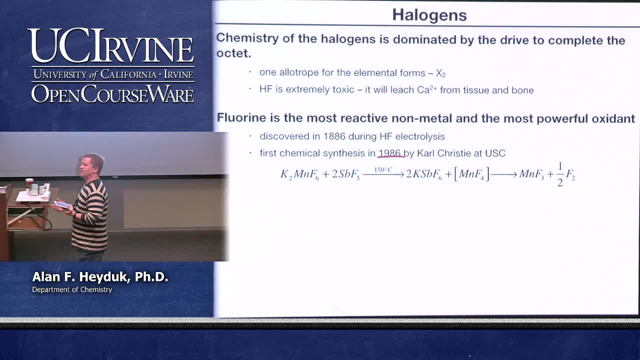 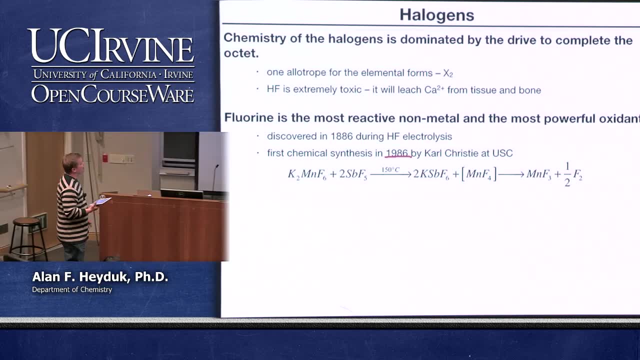 This is an element gas that we had to wait until 1986 to make And you can see. So you can see that it was made in a pretty unusual way. So you can start with this: dipotassium manganese hexafluoride. 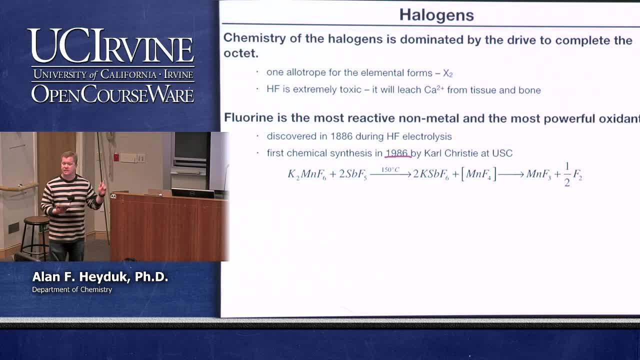 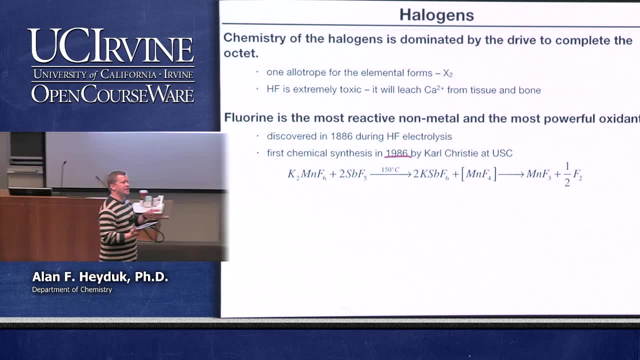 And you react it with anemone penefluoride. We've already seen the anemone penefluoride. Does anybody remember where? Superacids, Superacids Exactly. SBF5 is an incredibly strong Lewis acid. 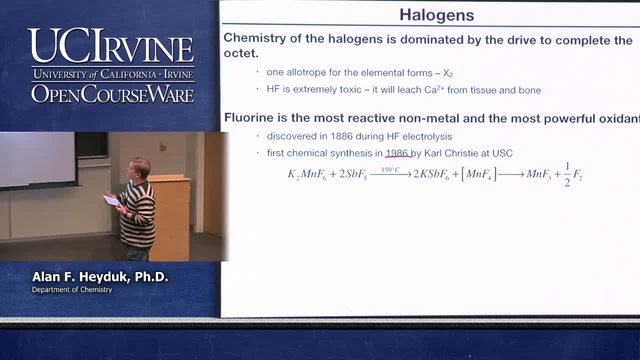 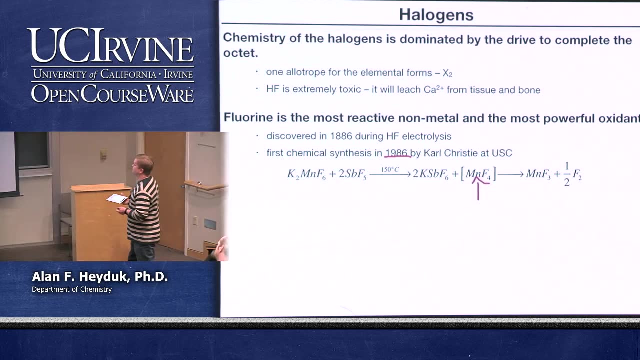 And it really, really wants another fluoride anion. So what happens here is this: equivalents of SBF5. come in and take two fluorides from the manganese and make this metastable manganese tetrafluoride, which then reacts in a bimolecular way to spit out fluorine gas, and one equivalent of manganese. 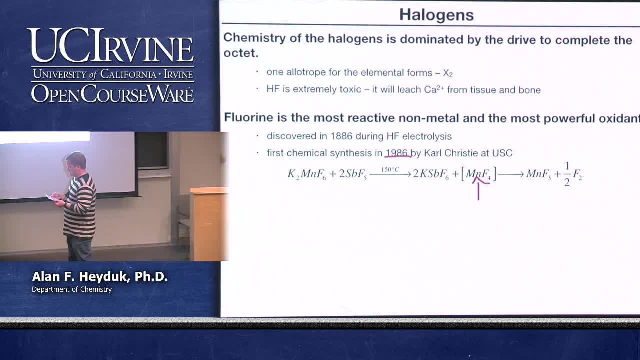 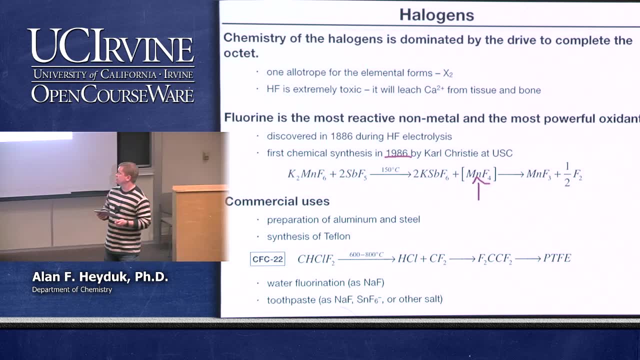 trifluoride. Pretty cool reaction, but it's just crazy to me that we had to wait till 1986 to make it Now. fluorine has lots of industrial uses. We use it in production of metals like aluminum and steel. It's a critical component in 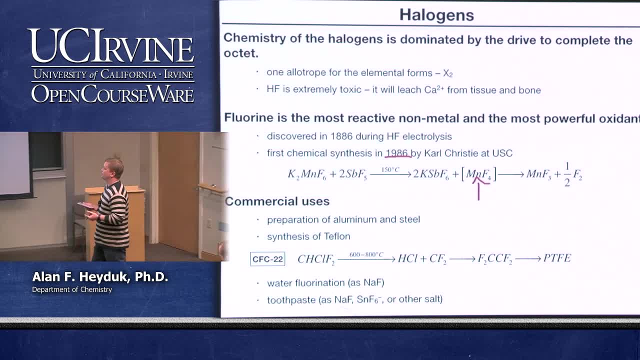 Teflon. That's what gives Teflon its slippery properties, and so the other thing is this species right here. Anybody want to know why you should care about that. It's a chlorofluorocarbon and, in particular, this was the the real. 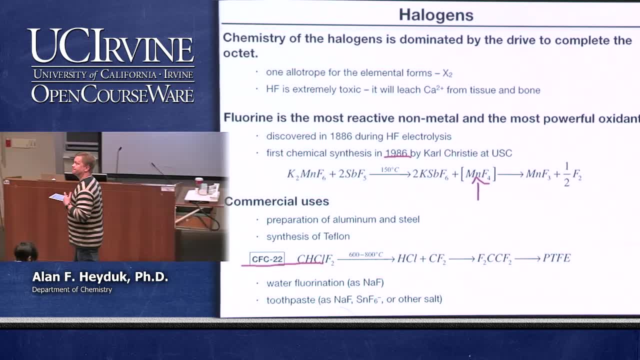 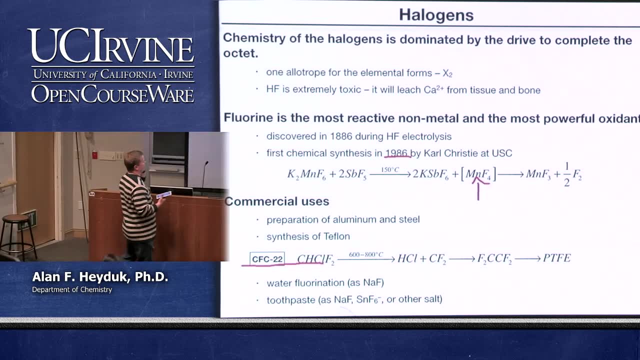 baddie that was depleting the ozone layer, CO2. CFC 22.. The reason it's named 22 is DuPont came up with this crazy naming scheme where the 2 in the ones position corresponded to the number of fluorines. 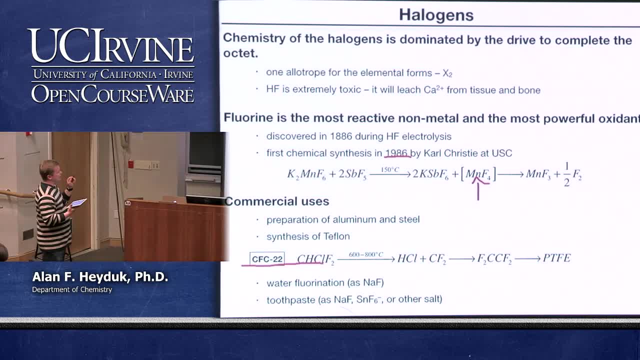 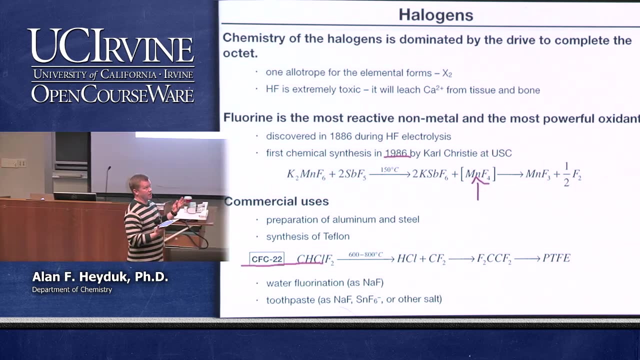 in the CFC, The 2 in the tens position was the number of, I think, chlorines plus 1, and then the fact that there's nothing in the hundreds position tells you that there's only one carbon atom. So the number in the hundreds position is the. 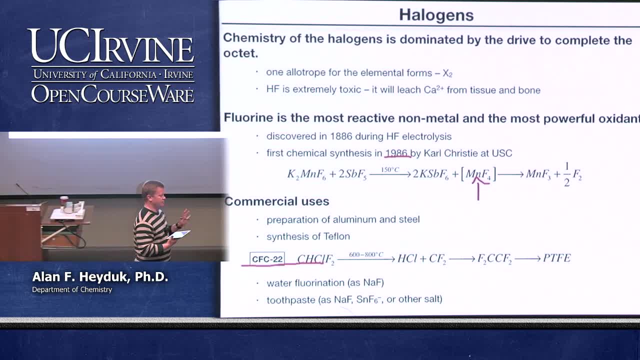 carbon atom. You're right, The carbon atoms minus one, It's just crazy, crazy numbering scheme. but this one is particularly reactive and you can see that from this reaction, even You heat it up to 600 degrees Celsius. I mean, that's a pretty unusual reaction. right to take a methane. 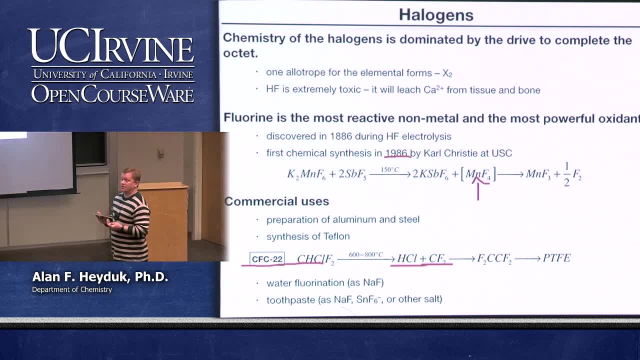 analog. heat it up and spit out the carbene. You actually eliminate HCl, you make the CF2 carbine which then dimerizes, polymerizes to make tetrafluoroethylene Turns out. at DuPont they accidentally discovered Teflon by having a cylinder of tetrafluoroethylene around that spontaneously polymerized and they ended up. 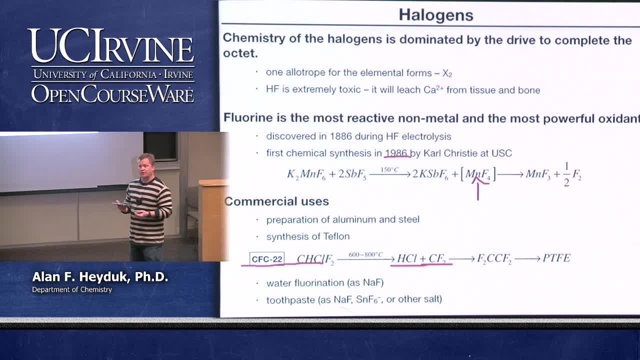 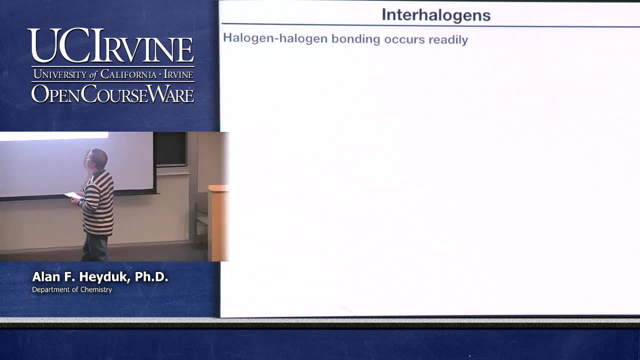 with this mass of very slippery, unreactive plastic that now coats all of our pots and pans and this and that and the other thing. So fluoride is used in water. fluoridation, Of course, we all know it's in our toothpaste as well. Interhalogens, So we always think about F2, Cl2, bromine and so on, and 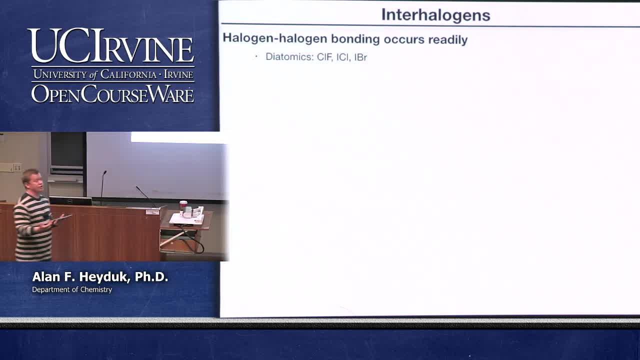 so forth. You can get interhalogen bonds So you can make the diatomics like the chlorine-fluorine bond, the iodine-chlorine bond, the iodine-bromine bond. Those are all good, They follow the. 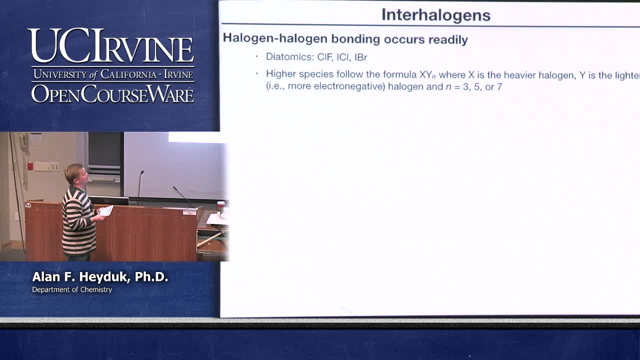 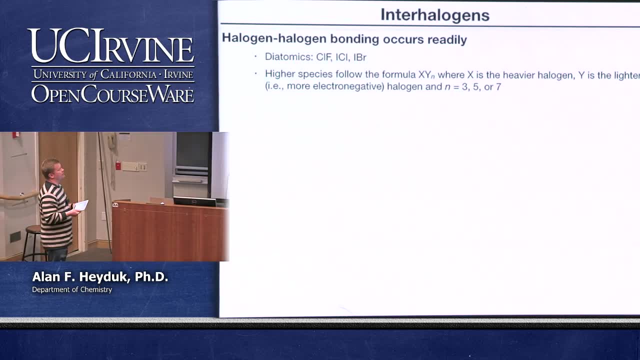 standard, The ordering XY to the N, where X is the heavier halogen, Y is the lighter halogen and then N can be, well technically, 1,, 3,, 5 or 7.. Okay, so always the lighter halogen is the one that has the greater. 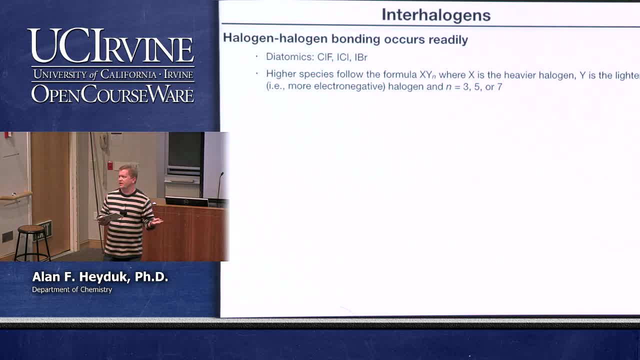 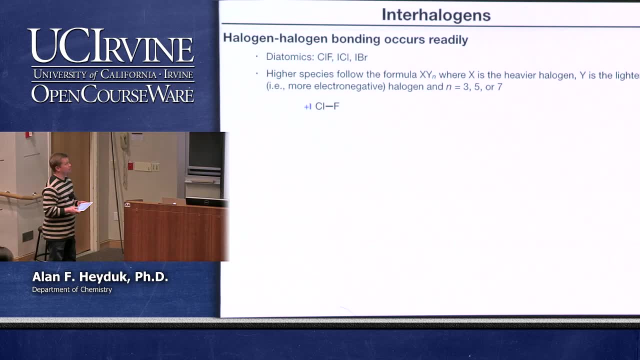 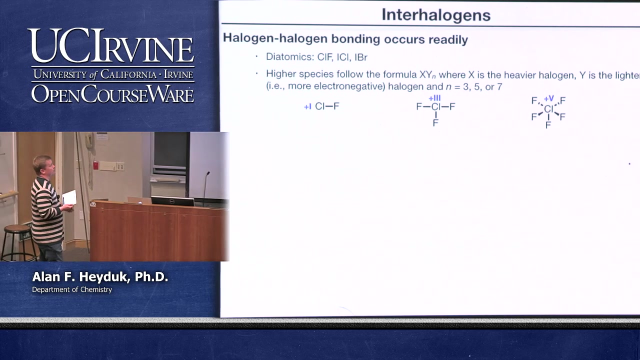 number Y, electronegativity and oxidizing power. So if we take chlorine and bond it with fluorine, we can make chlorine in the plus one oxidation state. We can take chlorine and make it in the plus three oxidation state by adding three fluorides to it, or we can make: 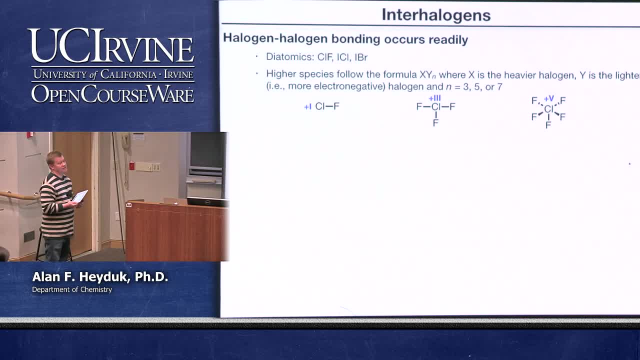 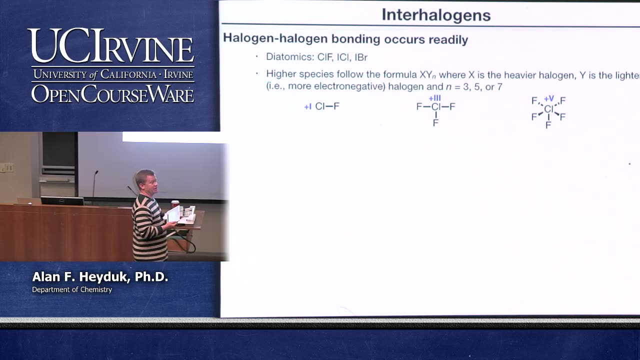 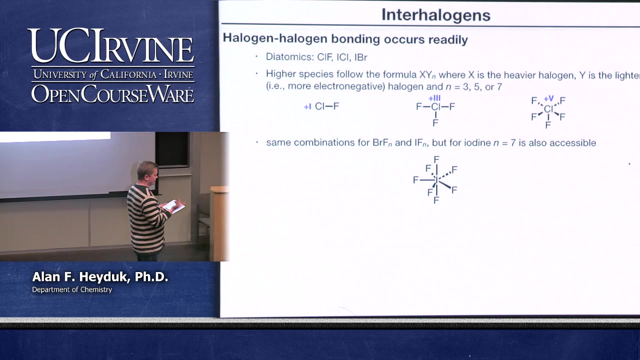 chlorine pentafluoride plus five oxidation state. Can I drive home the point again that fluorine is a powerful oxidizing agent? Okay, it's taking chlorine, the third most electronegative element on the periodic scale table, and taking it up to the plus 5 oxidation state. That's as far as you can. 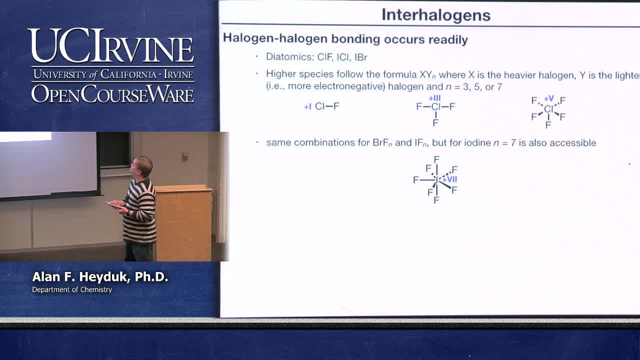 go with chlorine. but if you go, if you take, if you switch to iodine, you can then oxidize it all the way up to the plus 7 oxidation state. you get this trigonal pentagonal bipyr or this pentagonal bipyramidal structure. So you 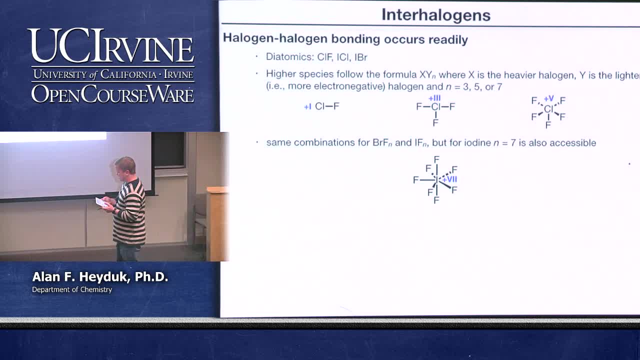 have five fluorines in a in the equatorial plane and two axial. Anybody want to hazard a guess as to what the point group is? Oh, forgot about that. huh, D5H? yeah, right, because you have a mirror plane. that's defined by the equatorial. 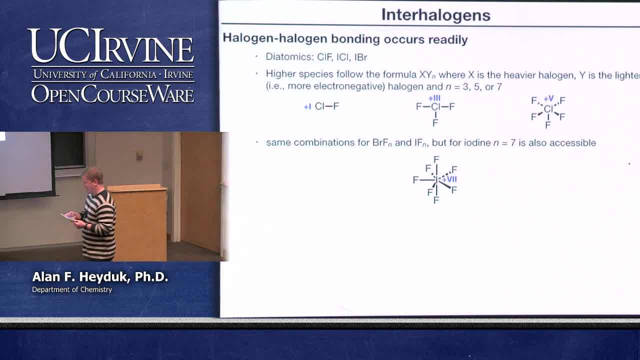 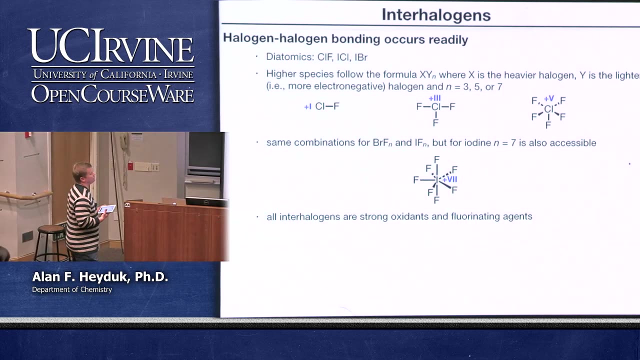 plane. You got half of those 20% points back. Okay, you. as you might suspect, even though fluorine can oxidize these halogens and reach these ridiculously high oxidation states for the halogen atoms, they're all still very reactive and they tend to be fluorine transfer. 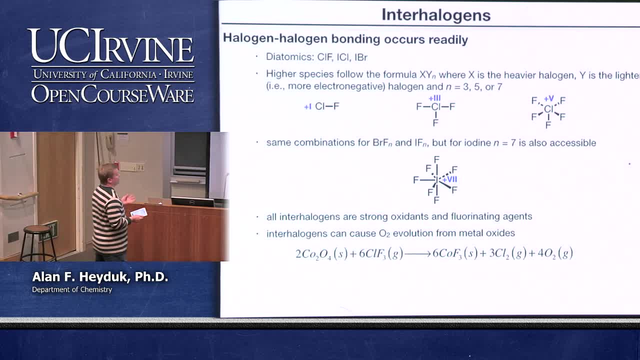 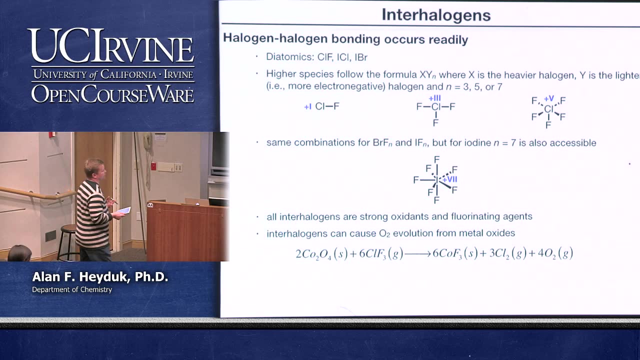 reagents, And so in some cases you can even use these inner halogens to oxidize metal oxo complexes and give off oxygen. So cobalt oxide reacts with the chlorine triphlorine Gas. you'll end up with cobalt fluoride as the cobalt containing byproduct. You 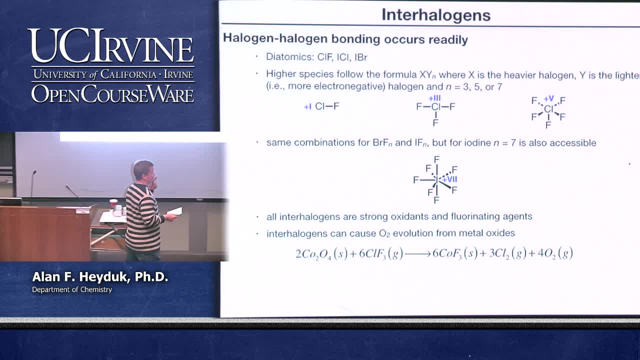 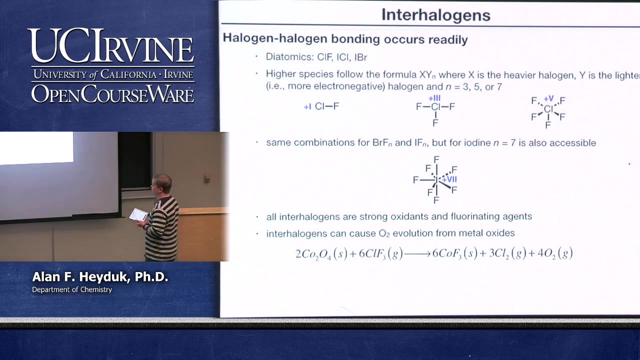 evolve three equivalents of chlorine gas and four equivalents of oxygen gas. This is some pretty nasty reaction conditions and if you think about the fact that chlorine right is typically used as a reagent itself to oxidize and destroy other as basically in sanitation applications, The fact that you're producing it really is a it's a pretty spectacular reaction. 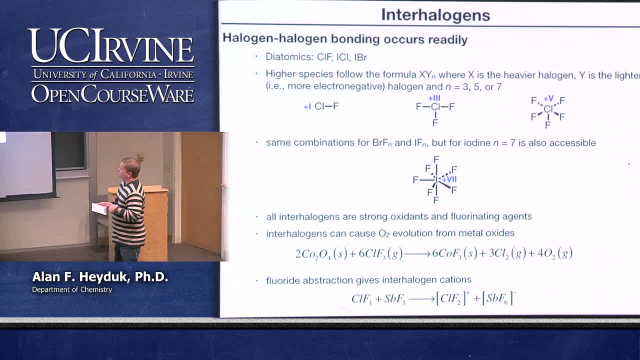 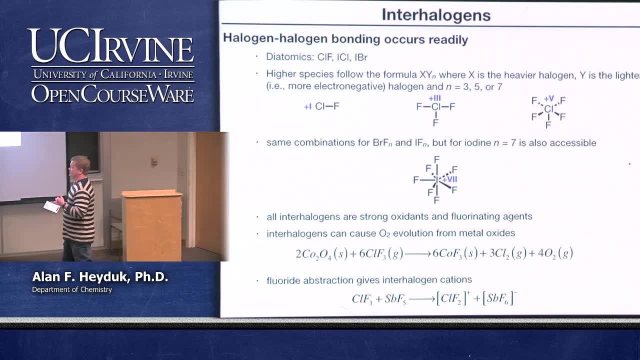 As if that wasn't enough, you can even make cations of the halogens. This is another one that just it's like you know you do chemistry all your life and you think you have a good feeling for what can be done, But the fact that you can make chlorine di fluoride cation. I mean that to me, is about as exotic as a cation can possibly look. right, We're taking elements that typically like to be negative anions and we're turning them into cations by combining multiple. It's just, it's crazy. There are also oxo anions of the halogens- Well, all of them except fluorine. OK, as I mentioned, oxygen is the second most electronegative element on the periodic table, And so it can oxidize various halogens and it forms an important class of anions. So there's a whole host of oxo anion acids. So here we have. 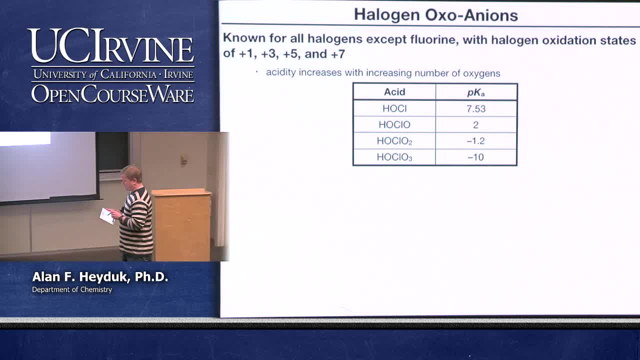 the acid of hypochlorite, chlorite, chlorate and perchlorate. And you can see that as we add more oxygens to the chlorine, the acid becomes stronger and stronger and stronger. OK, again, this should make sense to you, because as we add more acids, the chlorine oxidation. 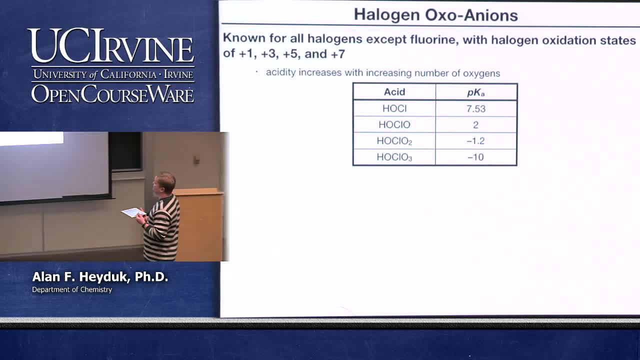 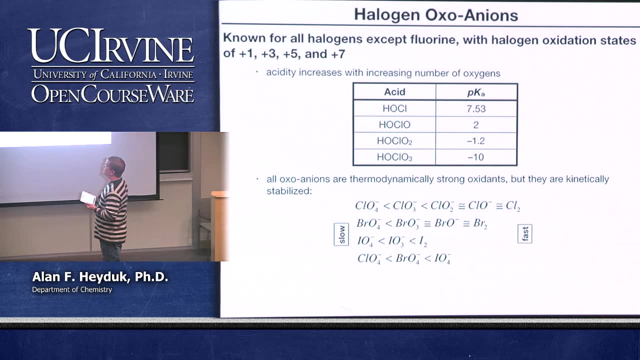 state is going up and the ability of the, of the molecule or of the anion to hold onto that protein proton is going down. So all of these are very strong oxidants, but there's they have different kinetic stabilities, So the most oxidizing thermodynamically is probably. 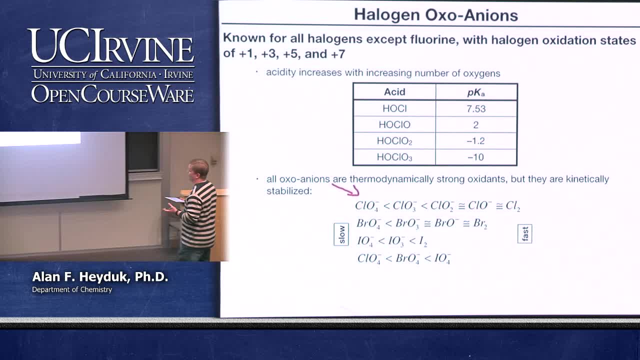 perchlorate. OK, it's chlorine. in the plus seven oxidation state It's got four oxygens. Yes, it's got one minus charge, but that's still chlorine plus seven. Thermodynamically we go down perchlorate to chlorate, to chlorite, to hypochlorite. 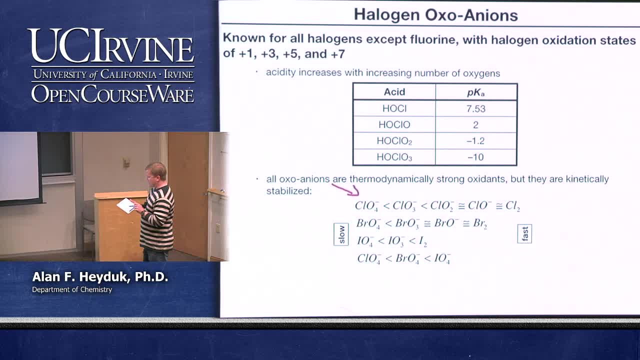 And then you have chlorine, but the kinetics of the oxidation, So in other words the speed at which they, or the ease with which they start their oxidation reaction, is inverse. So chlorine is kinetically the fastest oxidant, Hypochlorite the second fastest. 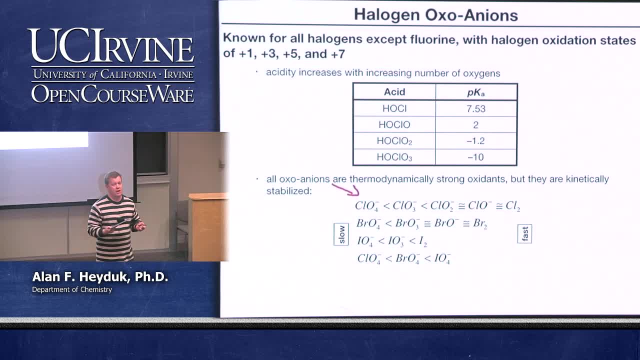 Anybody know what hypochlorite is Bleach? So when you put bleach in the laundry, what you're actually doing is you're putting an oxidant in there that oxidizes up any organic compounds that are causing stains, And when they get oxidized, it destroys them and they become colorless. 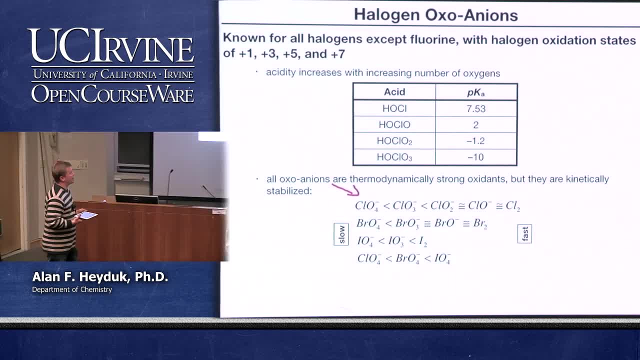 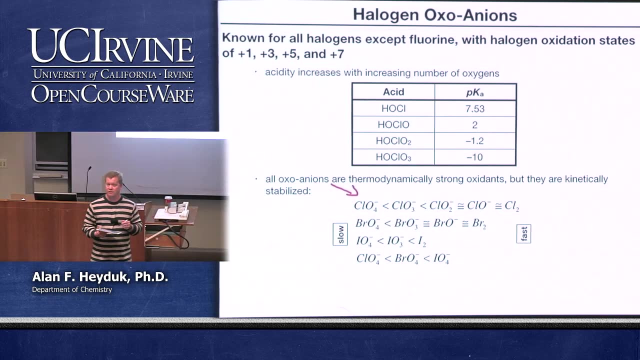 So you're doing oxidation reduction chemically? OK, So you're doing oxidation chemistry by adding bleach to your, to your laundry. For those of you that do undergraduate research, you may. you do electrochemistry. you may prepare salts. Be, if you haven't been told this, be exceptionally careful if you're using perchlorate counter anions. 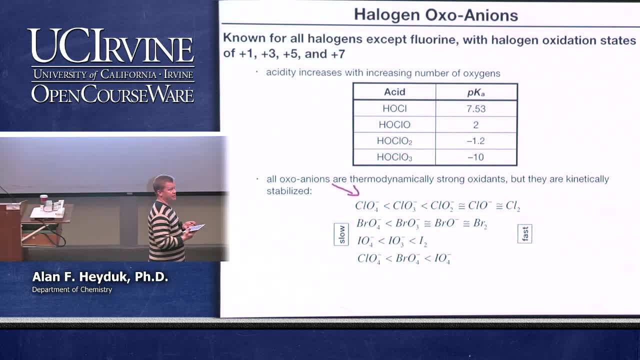 OK, because again, they're very, very powerful oxidants, but kinetically stabilized. So they'll sit there and sit there and sit there and be happy, And then, if you're not careful, if you do Something wrong, like grind it with a metal spatula, you'll catalyze the oxidation reaction. 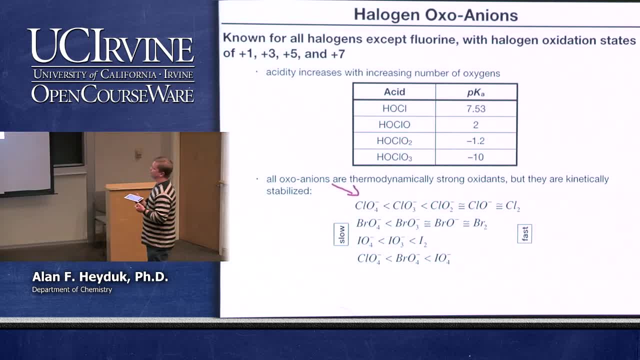 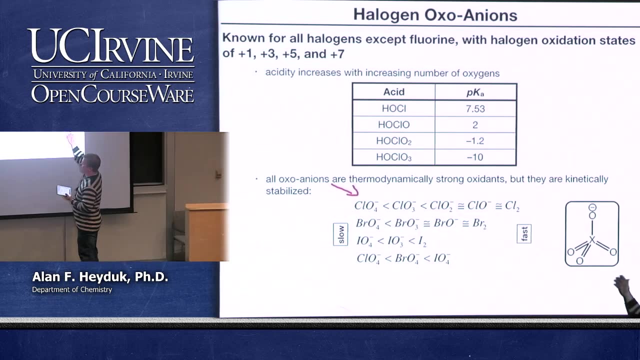 and they explode, OK, So people have lost fingers to perchlorate anions, So you have to be real careful Now. as for this kinetic stability, Again, it probably makes sense if you look at the structure. So with the perchlorate or the perchlorate or the perchlorate, we basically have a tetrahedral. 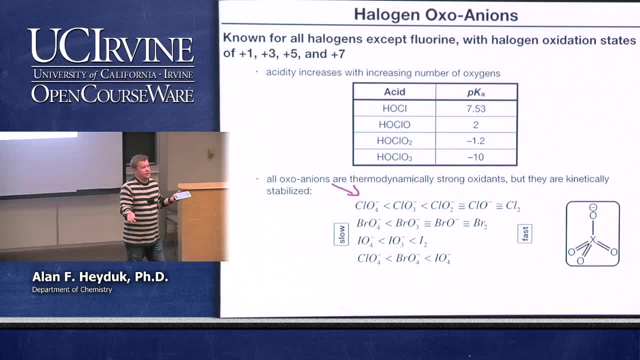 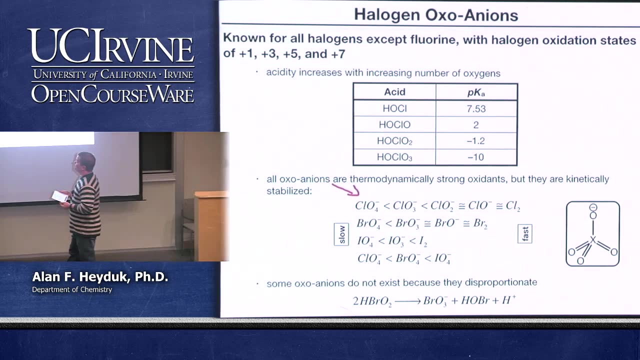 structure Looks the same in all three dimensions. You get resonance structures where you can move the double bonds around and you basically stabilize it through this idea of resonance That you'll notice from this table that there are some oxo anions that are missing. 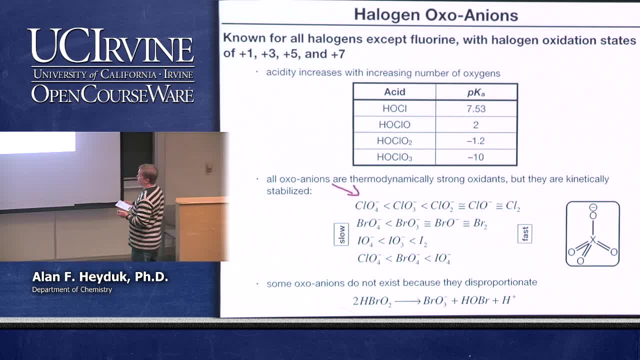 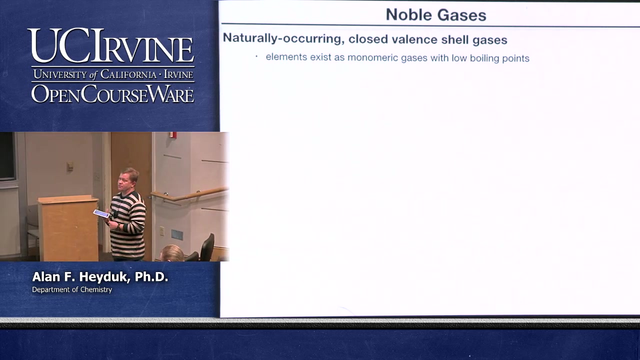 For instance the, the B, R, O, 2.. So that's bromite is missing and that's because in aqueous solution it disproportionate to the bromate And the hypo bromic acid plus a proton. OK, last of our p block march the noble gases. boring, don't do anything. 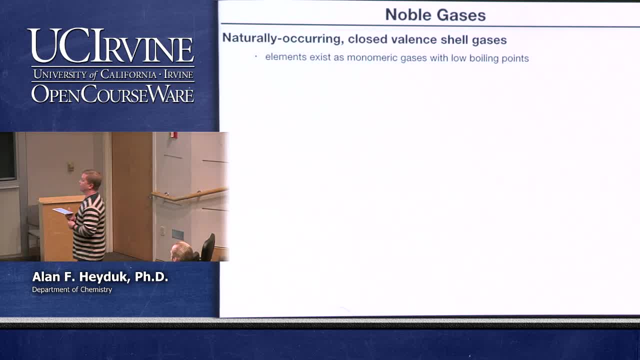 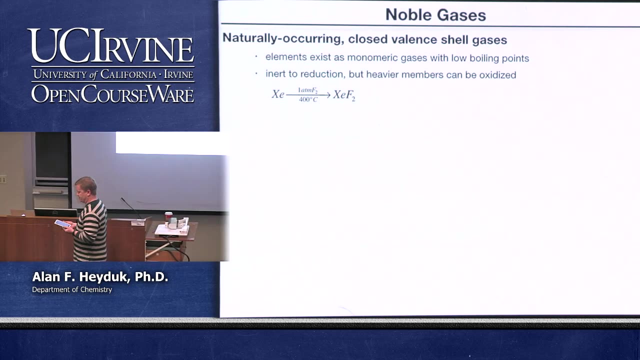 They may be the only set of elements that's. that's more boring than carbon, right? We all know they're perfect spheres. they exist in their elemental forms, as the pure, as as single atoms with really low boiling points. It turns out. again, as many of you probably know, they can be oxidized. so if you take xenon, with, oh surprise, the most oxidizing element on the periodic table. You can break up that noble gas configuration, and so xenon with one atmosphere of fluorine at four hundred degrees C gives you xenon di fluoride, great fluorinating agent. If you need to do, it's a. it's a very volatile solid, but if you need to deliver an equivalent. 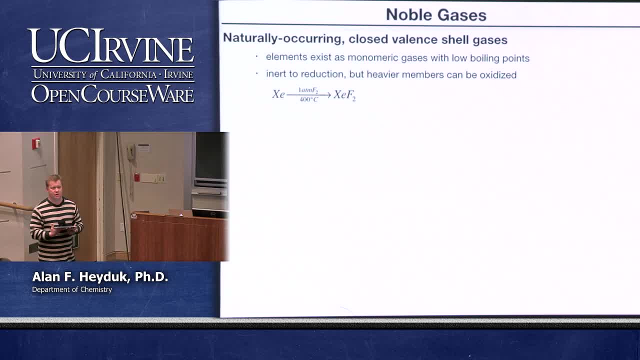 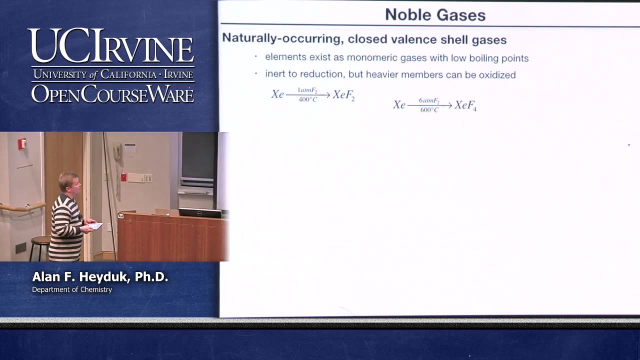 of fluorine It. You pull out your gas burette and measure out this really toxic gas. You can oxidize the xenon up if you, if you heat it at extra pressure of fluorine and heat it to six hundred degrees C, you can get the xenon tetra fluoride. And if you go up to sixty atmospheres of fluorine gas, you can get xenon hexa fluoride. OK, so this is now a noble gas in the plus six oxidation state. I wouldn't want to put a vial of it in my back pocket. 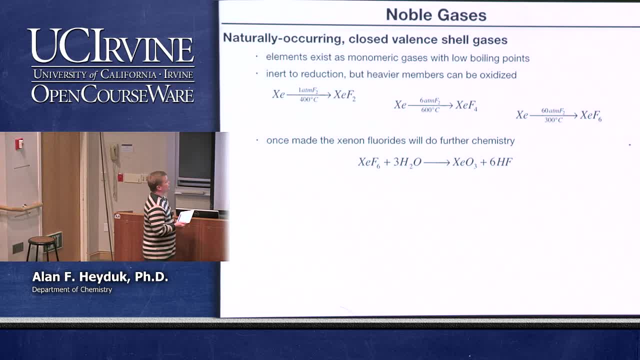 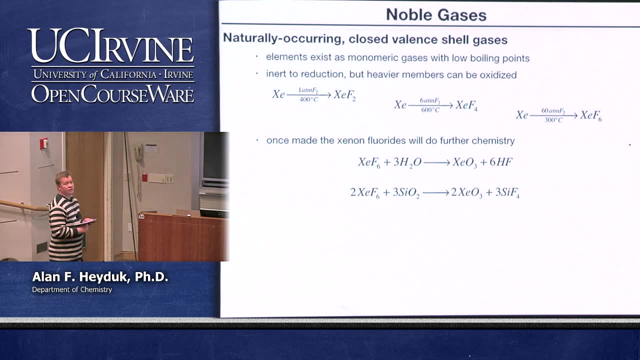 These fluoride complexes of xenon will do other chemistry. so if you take xenon hexa fluoride, put it in water. you can basically hydrate off the the HF and make xenon trioxide. There's one for you. Why does that reaction matter? 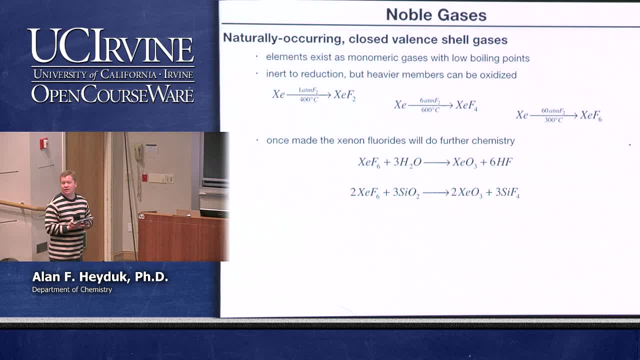 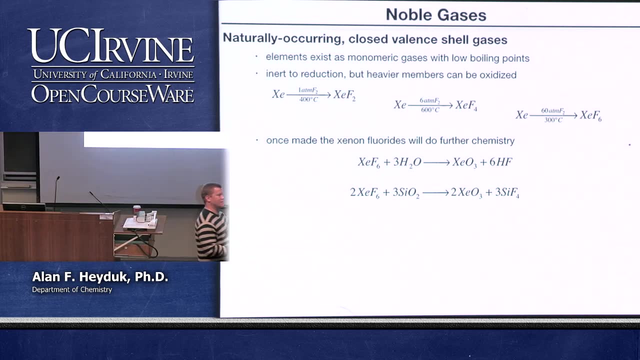 Xenon, hexa fluoride plus three, Silicon dioxide, Silicon dioxide. What's the lesson there? Don't put it in your glassware, right? So literally, what this is doing is it's etching glass. it's pulling silicon dioxide molecules off of the surface of the glass and making silicon tetra fluoride. OK, have I mentioned that these sorts of fluoride complexes are very, very oxidizing, very reactive. Yeah, OK, xenon trioxide is explosive, so don't go make it in the lab and isolate it. but the others are more stable. Xenon trioxide is kind of special that way. 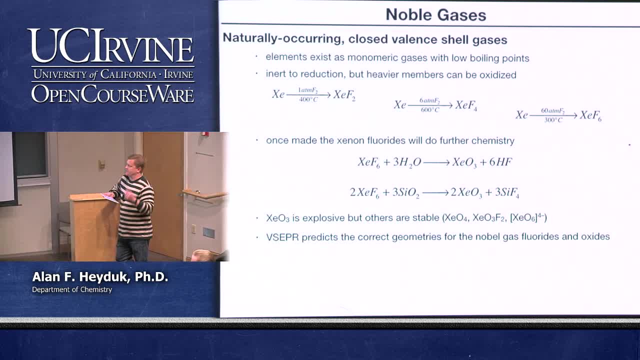 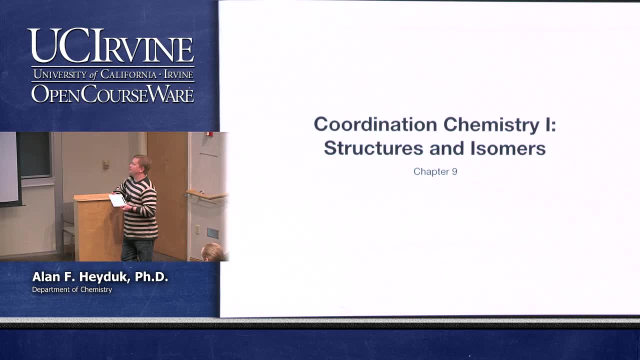 And for all of these VSEPR rocks, it always gets the right geometry for these noble gas fluorides and oxides. The end of the p-block elements. The end of the p-block elements. Now you know it's, it's, trust me. I know that when we're going through that stuff it's hard. 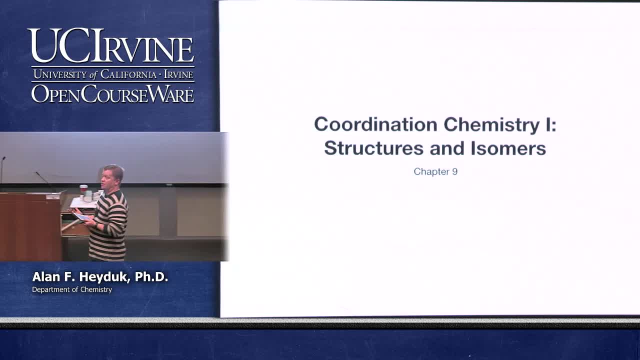 to sit there and listen right, and I know it's hard. It's even harder to read the chapter and to figure out what you need to know for the exam, but at the same time, that kind of descriptive chemistry. that's where you get a real appreciation. 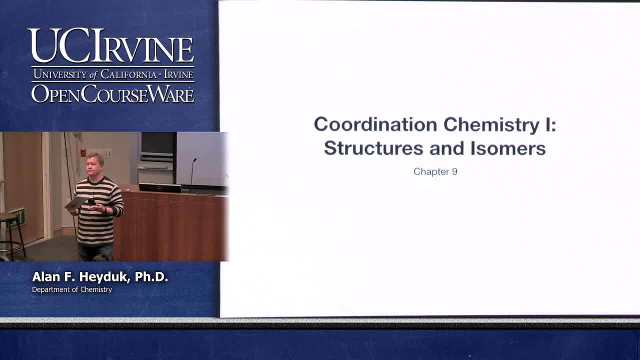 for where chemistry is used in the real world. Right, What we use different You know. These are the main uses of different elements, different kinds of compounds. These are the kinds of things that you need to know so you can go out and amaze your friends. 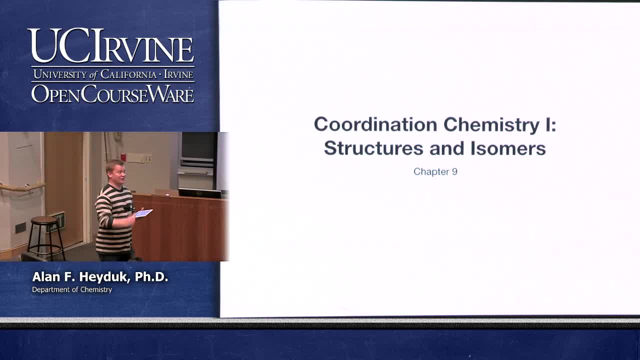 Right, Like you got used to, I know what that's used for. That's how we prepare aluminum: blah, blah, blah, blah, blah. And then everybody goes: oh you're so smart, You're a chemist, OK, OK. So coordination chemistry one. they ran out a good creative name, so we're going to go. 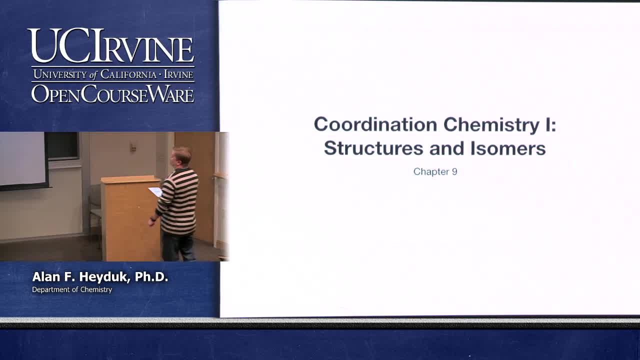 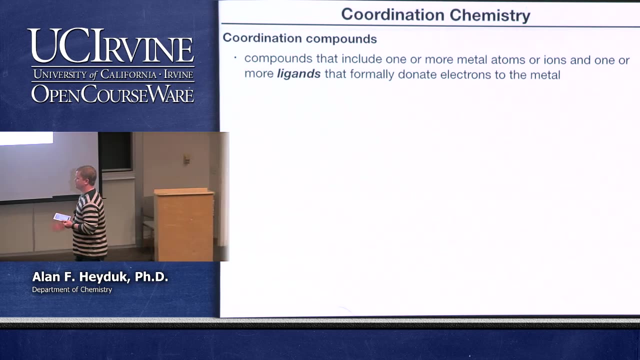 through chapters nine, ten, Eleven and maybe twelve, which are coordination chemistry one, coordination chemistry two, three and four. But we're going to start with structures and isomers. So what do we mean by coordination chemistry and why do we call it? why do we call them? 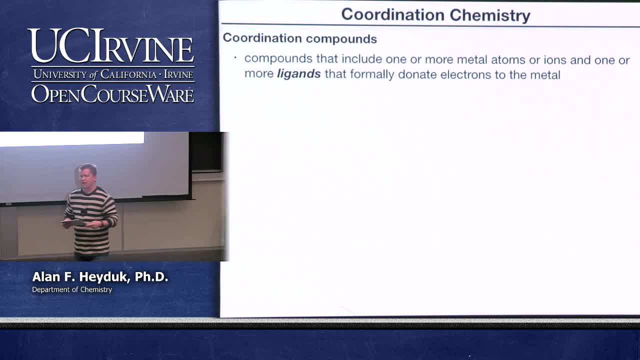 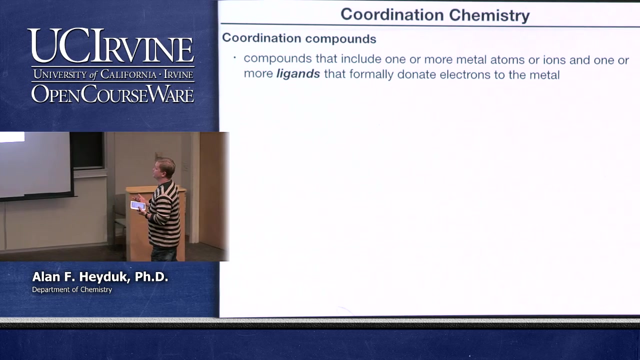 coordination compounds, And so it all goes back to acid based chemistry. Transition metals are almost universally considered to be Lewis acids, And the ligands that we coordinate to them are Lewis bases, And so we have a Lewis acid- Lewis base interaction. The ligands are the Lewis bases that are donating at least one pair of electrons to the transition. 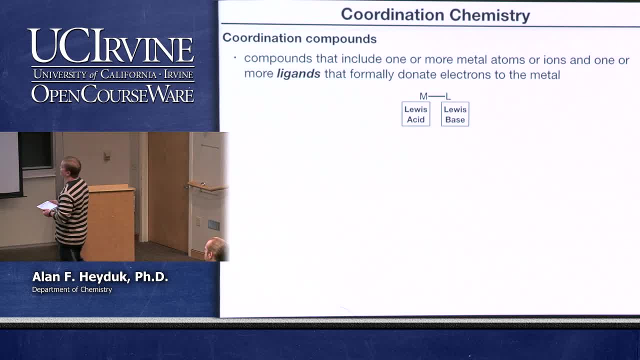 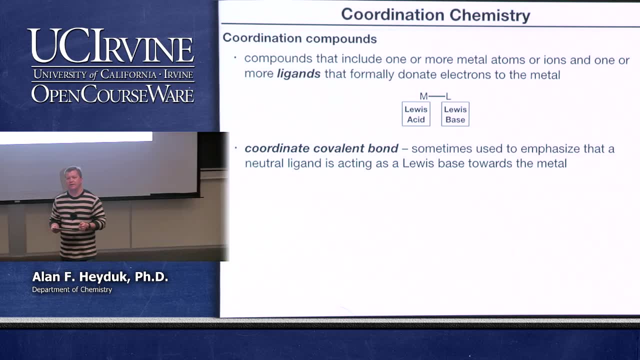 metal. Yay, This brings up the idea of a coordinate covalent bond. You will also hear this referred to As a dative bond. OK, It's a very specific type of Lewis acid, Lewis base interaction, And I'll highlight this. 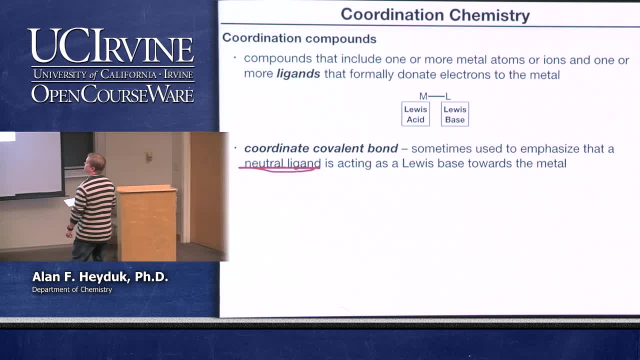 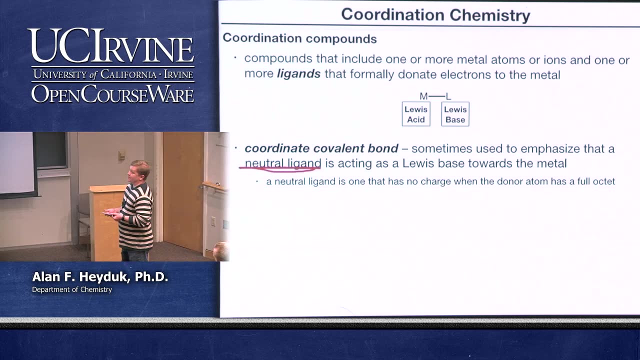 It's a coordinate covalent bond is highlighting that you're using a neutral ligand or a neutral loop. you're coordinating a neutral Lewis base to the Lewis acidic transition metal. OK, So a neutral ligand or a neutral base is one that doesn't have a charge when the octet is complete. 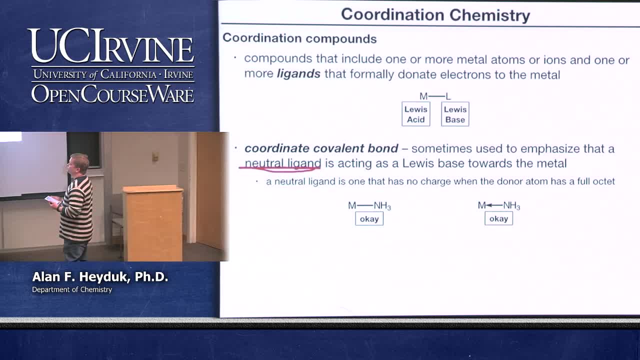 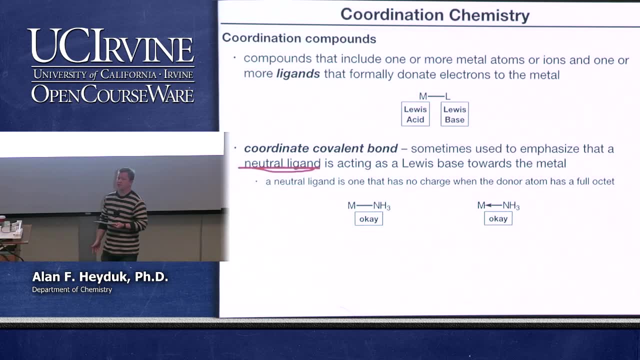 And so the reason that this idea of a coordinate covalent bond comes up is because you'll see something like ammonia. It's a great ligand for transition metals, Right, We know that ammonia is a good Lewis base, And so it stands to reason. if metals are Lewis acids, it should be a good ligand for for a transition metal. 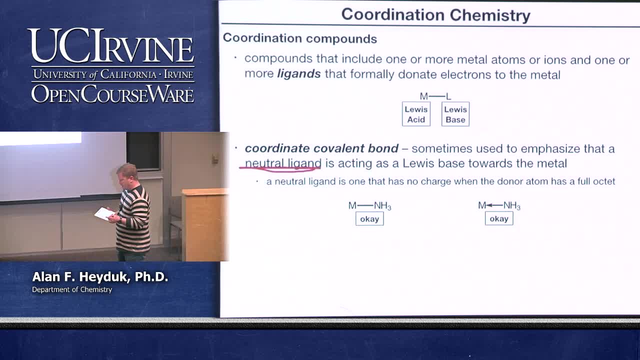 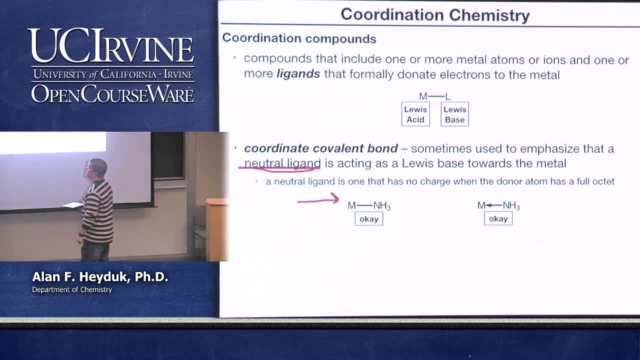 And so you'll see this written in two different ways. This is probably the most common ligand for transition metal. This is probably the most common Where you just have the normal kind of single line connecting the nitrogen to the metal center. OK, 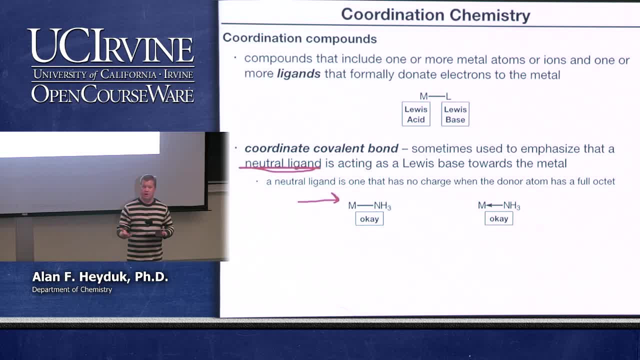 In Lewis structures. we know that that single line means that the two elements are sharing a bond and they have a sigma bond. OK, And that's fine. You'll also see it written, And this is really a more complete way to describe a coordinate, covalent or a dative type bond, because it's 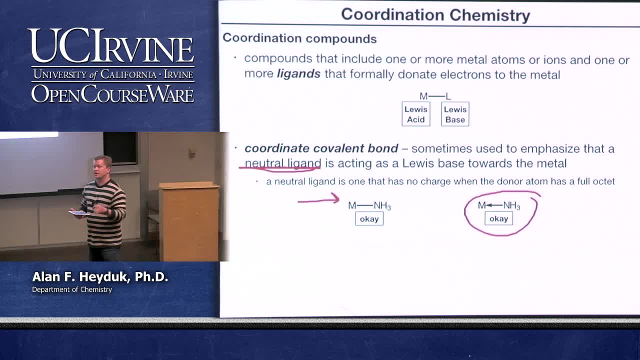 Emphasizing the fact that ammonia is a neutral Lewis acid. So basically what this comes down to is that arrowhead is a way to count electrons. It's keeping track of, kind of who those electrons belong to if everything is going to be neutral. 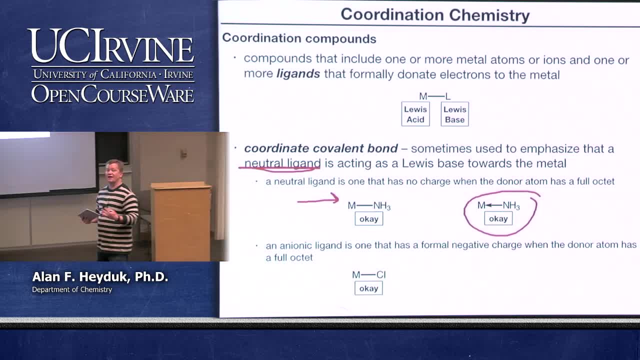 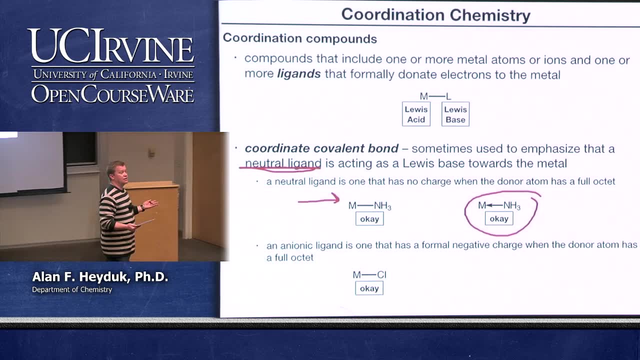 Now where you have to be careful is we also have anionic Lewis bases: Right Chloride. Right, Chloride is a Lewis base, but it's got a charge. It's also OK to write chloride with a single bond: Metal chloride interactions it's. they're sharing a pair of electrons. 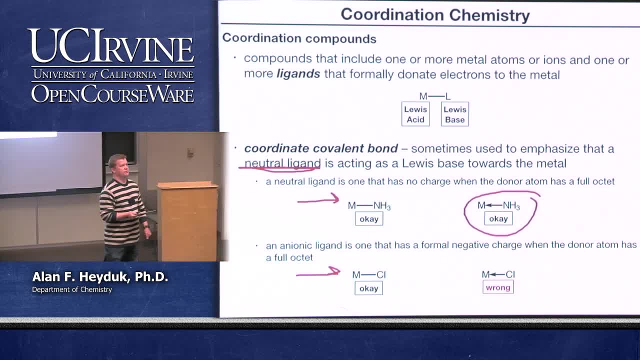 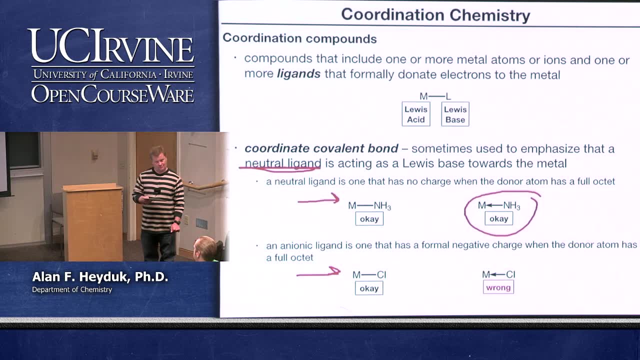 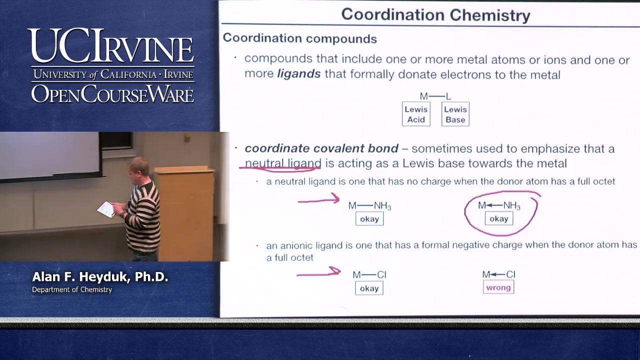 Do not ever do this, OK, I will hunt you down And throw dog poop on your front door or something In you know the flaming paper bag. It would be great. Do not do that, OK. Yuck Makes me very angry. 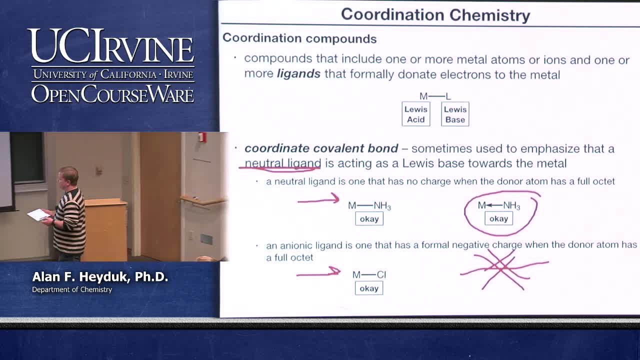 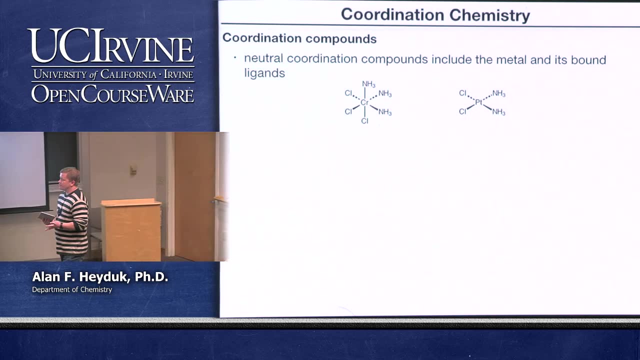 We on the same page, But this can be a very useful way of drawing bonds between neutral Lewis bases and Lewis acidic transition metals. OK, So a neutral coordination compound includes the transition metal and all of the Lewis bases that are coordinated to it. OK, 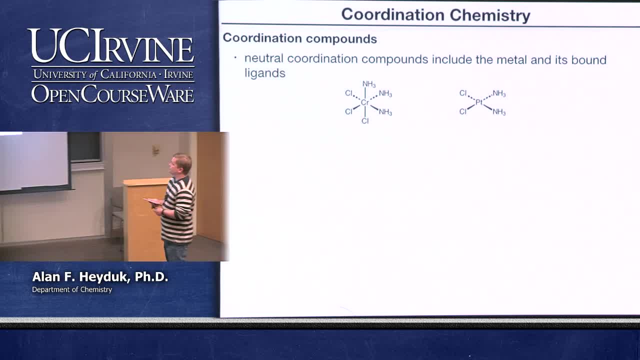 So we have two examples: The hexam, or triamine, chromium trichloride, Diamine, platinum dichloride. Anybody know what's so important about the molecule on the right Wrong Catalyst for organic reactions? That wouldn't be interesting at all. 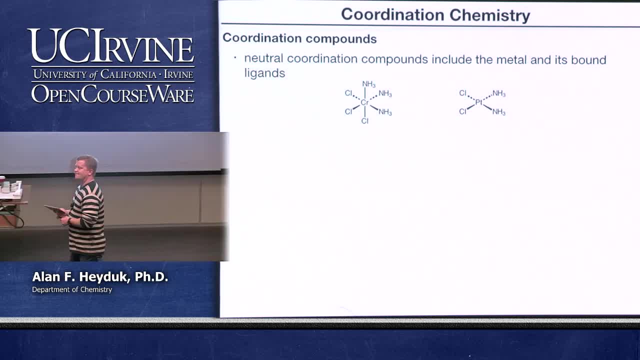 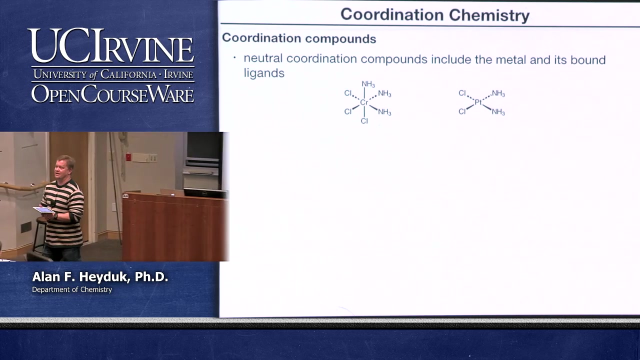 I'll give you its super secret name, or I should say common name, Cisplatin. How's anybody know? I heard it come from over there. Yeah, It's one of the most effective cancer drugs on the market. That's the drug that saved Lance Armstrong's life- for better or worse, depending on if you're. 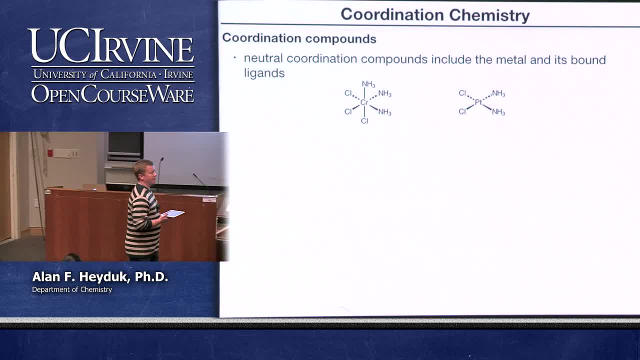 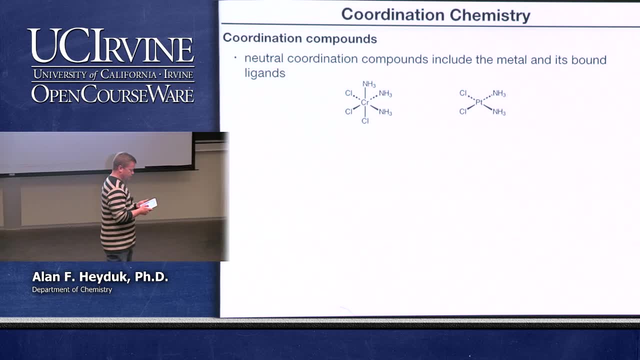 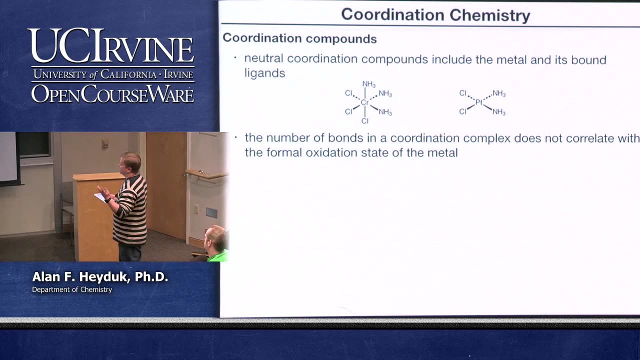 a cycling fan. OK, It's the absolute best drug for treating testicular cancer and several others. OK, We'll talk a lot about cisplatin, because it's a really interesting. It's a really good example for a lot of different coordination isomers and stuff like that. So the number of bonds in a coordination complex is not directly correlated to the oxidation state, the formal oxidation state of the metal, And so we can see that, based on even those examples above, So in this chromium complex the formal oxidation state of the chromium is plus three. 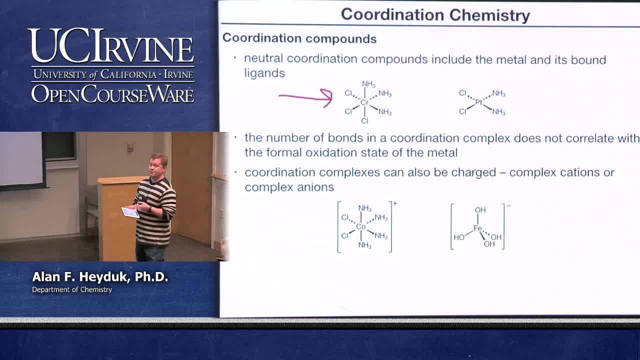 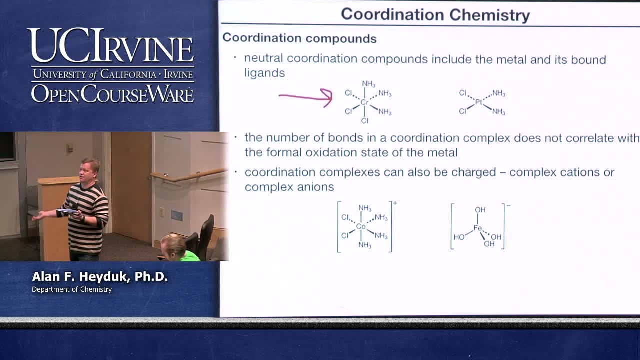 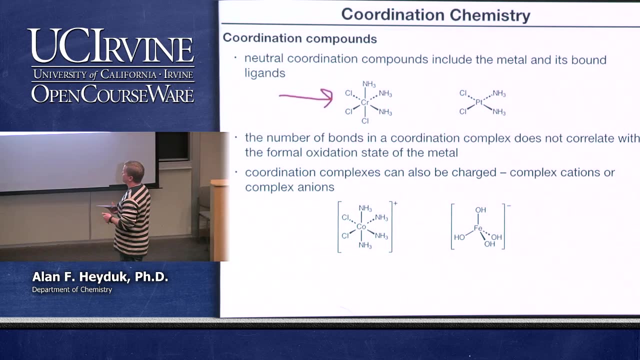 OK, In the case of the platinum compound it's platinum two, And so you might say: oh well, obviously the correlation is that the oxidation state is half of the number of ligands coordinated. That doesn't really work, But we'll talk a lot about oxidation states because it's one of inorganic chemists' favorite. 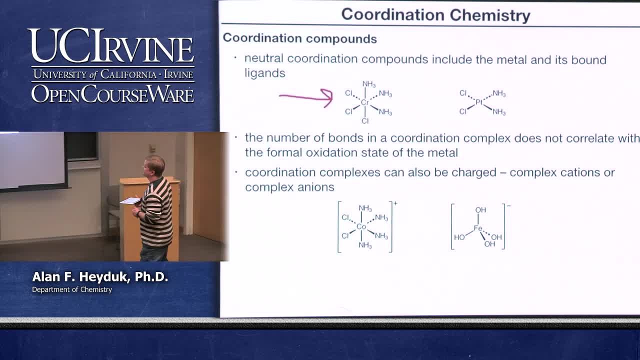 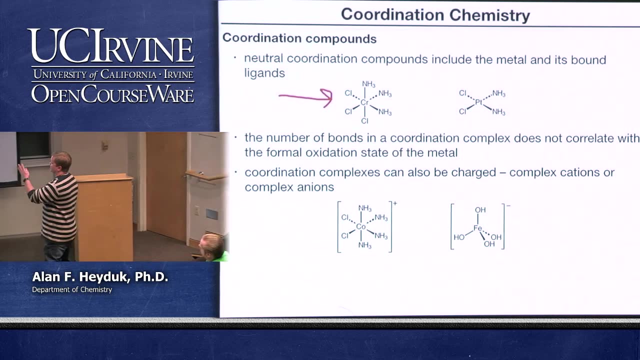 things to do is assign oxidation states to the transition metal in a coordination complex. Coordination complexes can also be charged. You can have complexes that are cationic or you can have complexes that are anionic. So here the example on the left. you can see what we have here. 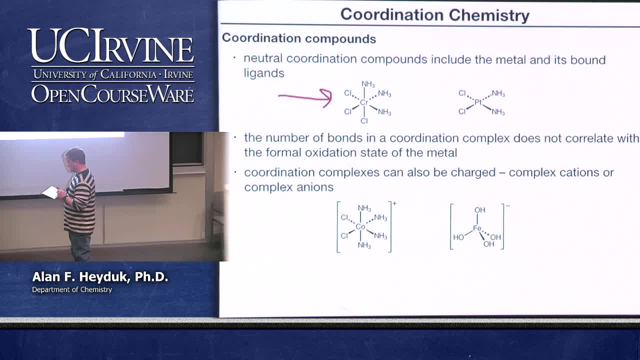 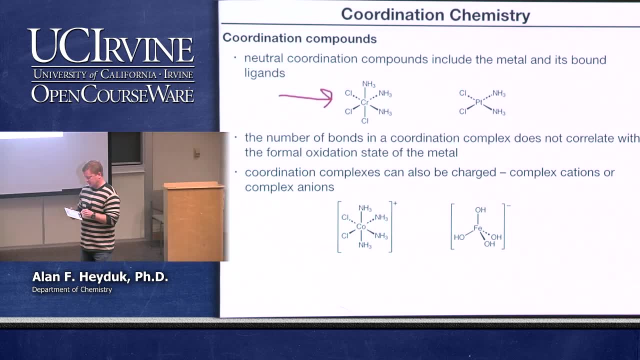 On the left you can see. what we've done is we've taken away one chloride and replaced it with a neutral ammonia. Now the complex is cationic. So in this species, this complex, the cobalt oxidation state is still plus, or in this case, 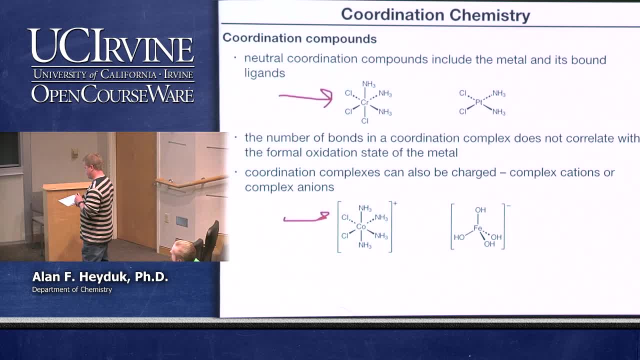 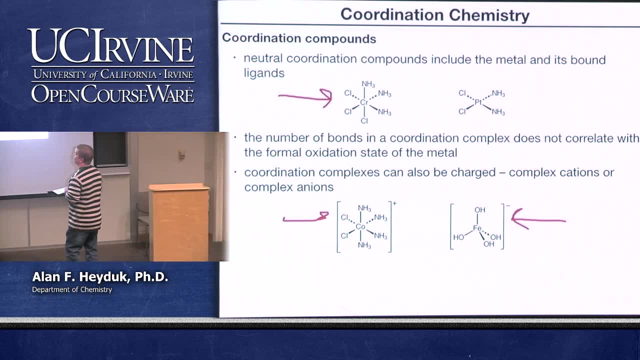 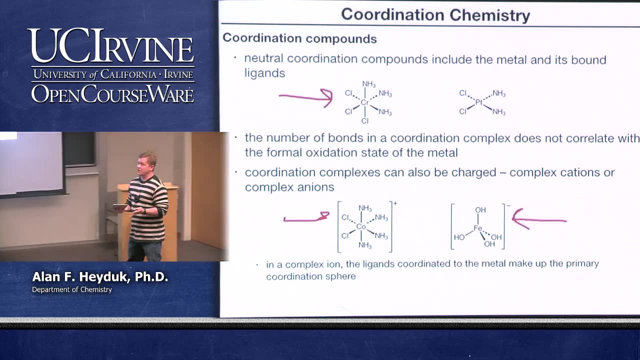 it's plus three, even though it's still a six coordinate complex. The complex on the right it's iron with four hydroxides. There's no anion. The oxidation state of that iron center is also plus three. So again, no correlation between the number of Lewis bases coordinated to a metal and 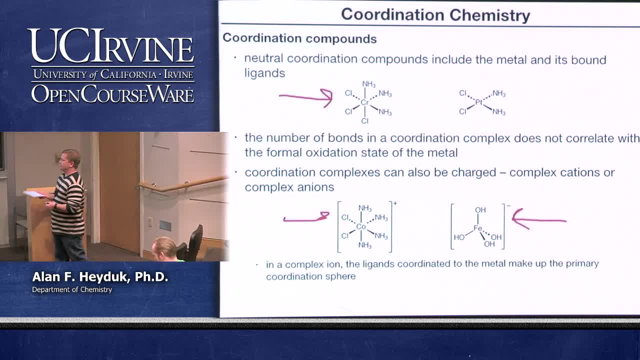 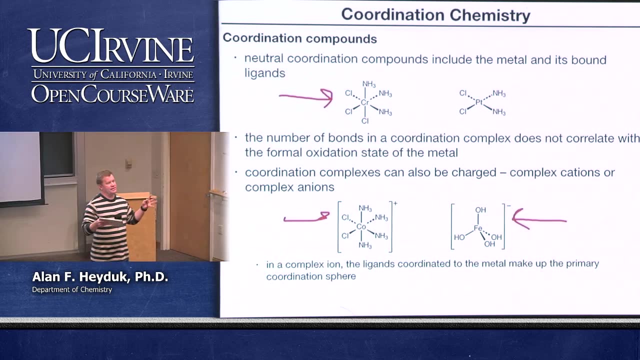 the oxidation state. When we're talking about these sort of complex ions, the ligands that are directly bonded to the transition metal make up what we call the primary coordination sphere. That primary coordination sphere that defines the geometry around the metal center is what controls its electronics and, in general, its reactivity. 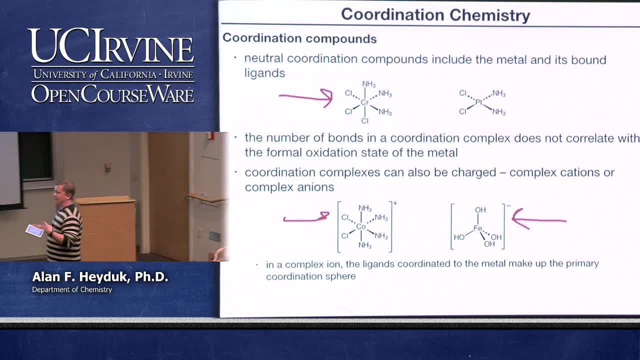 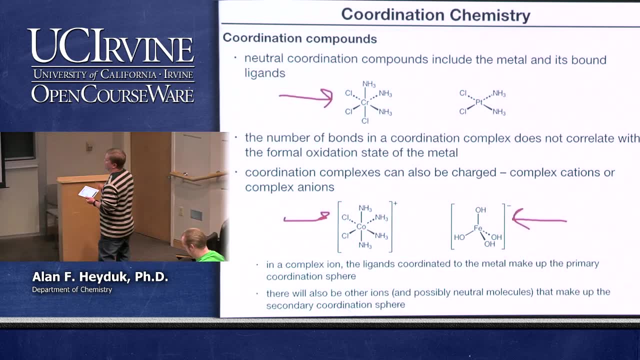 The counter anion or counter cation typically has much smaller effect on the overall reactivity or properties of the complex, And so again, there will be other. obviously, if you have a cation like this, you better have an anion around to balance it, because we can't put charged species in a bottle. 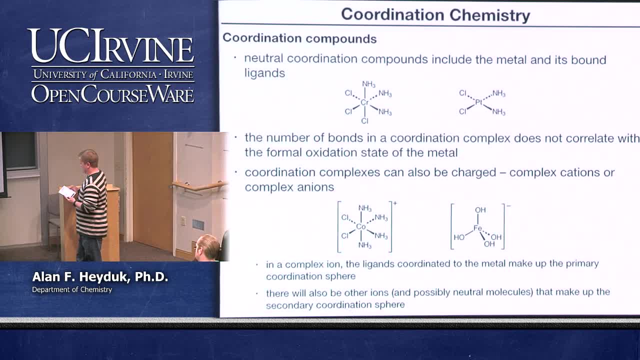 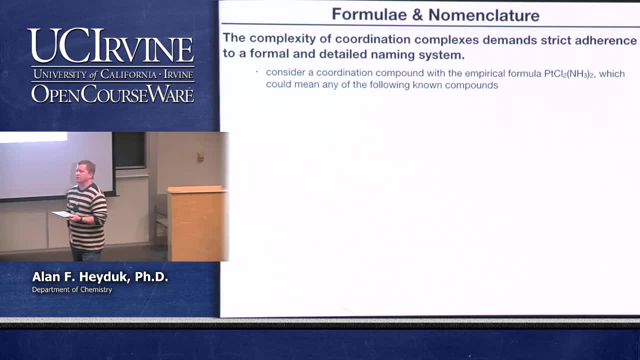 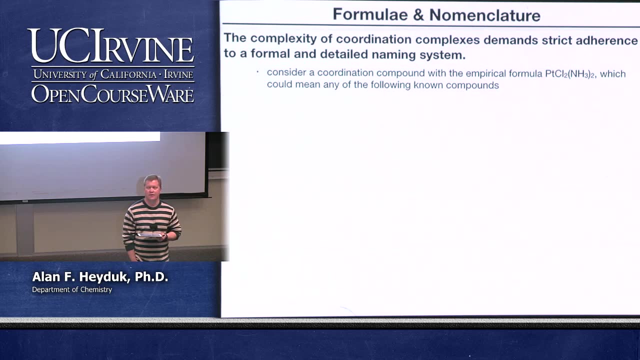 And they will make up part of what we call the secondary coordination sphere. Okay, So we know from Chem 51 that molecules can be really complicated, really complex, And, as such, naming of these molecules can be a real pain in the keister. 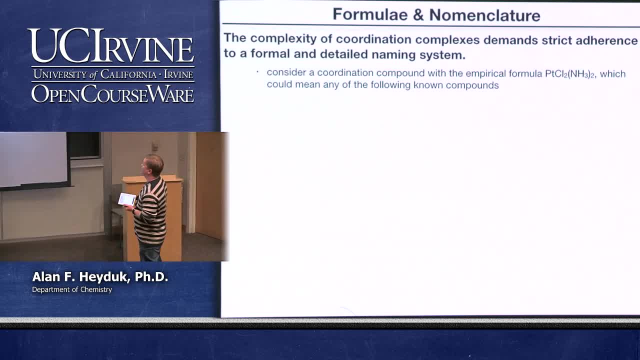 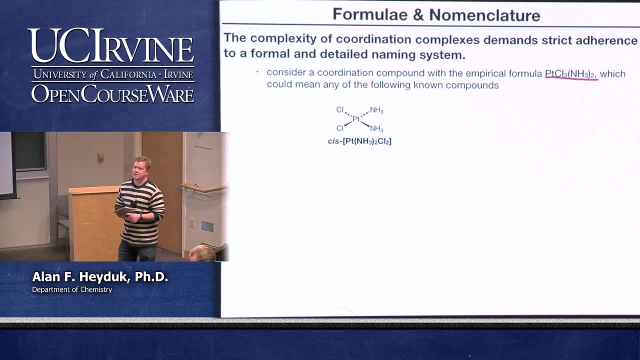 Okay, It turns out to be true for transition metal complexes, So we've already been introduced to the diammonia platinum dichloride complex. But the truth of the matter is it can mean several things. You're just given that formula. Well, it could mean cisplatin, the cancer drug. 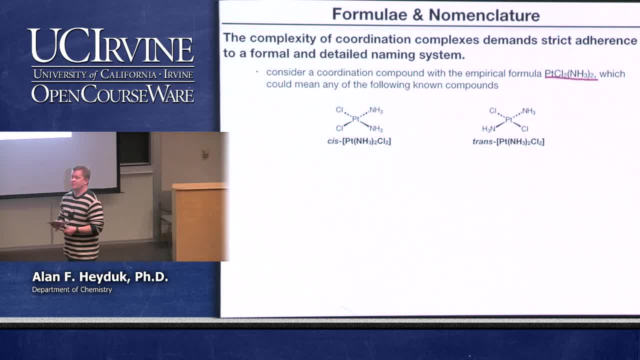 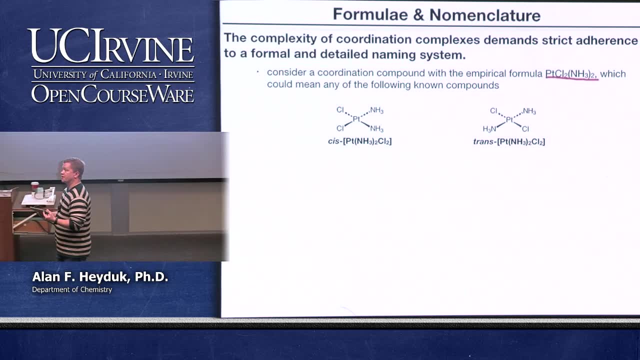 It could also mean transplatin. This platinum complex is square planar, So there are two different isomers, One with the chloride cis to each other related by 90 degrees, The other with them related by 180 degrees. Transplatin, not a cancer drug. 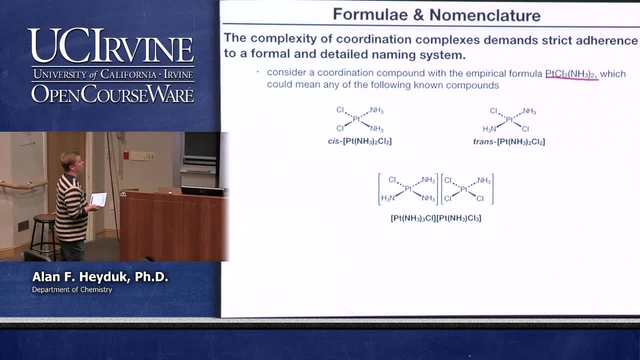 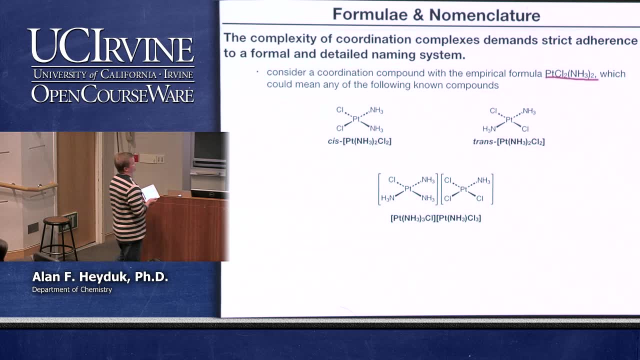 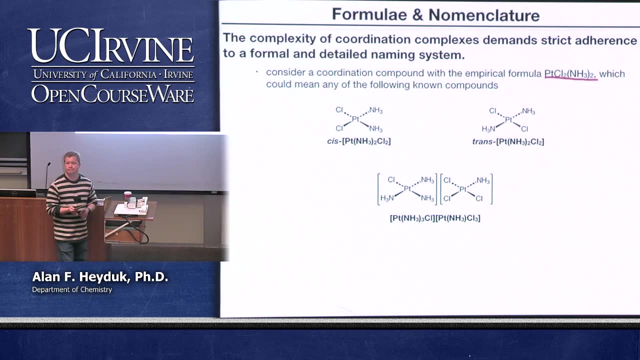 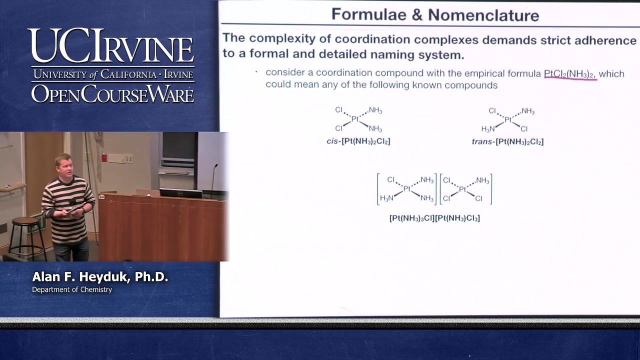 Just gives you heavy metal poisoning. Well now, that's weird. You can have the triamine platinum chloride cation with the amine platinum trichloride anion Has really the same right. If you write out the formula, it ends up being PTCl2, ammonia 2.. 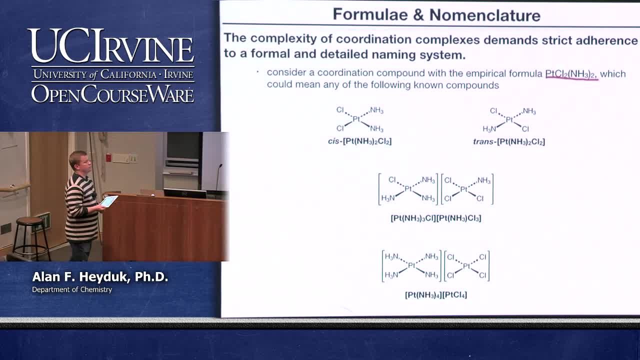 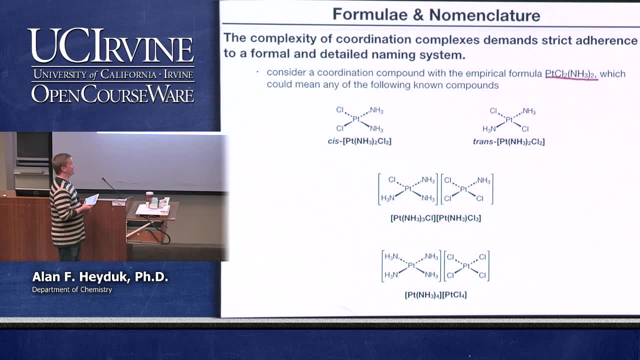 Well, now we're just being downright mean right To put all four ammonias on one- platinum- and four chlorides on the other. The platinum with four ammonias is plus 2.. It's a dicat ion. The platinum with four ammonias is plus 2.. 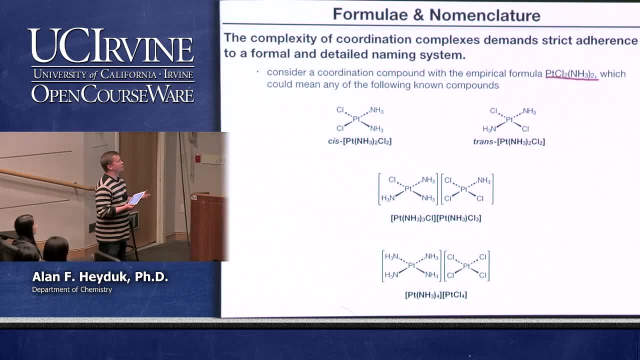 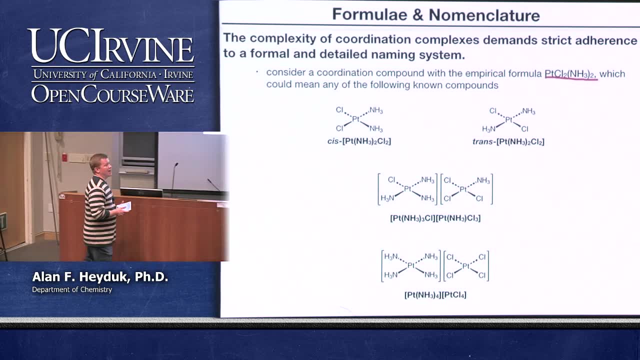 The platinum with four chlorides is a di-anion, So we have to have ways to name each one of these different isomers And identify them, so that when I give you the name of a platinum compound containing two chlorides and two ammonias, 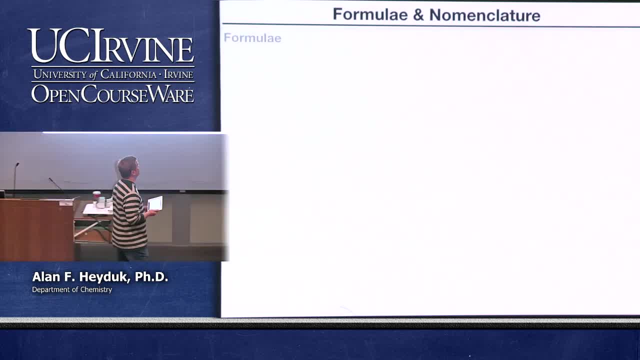 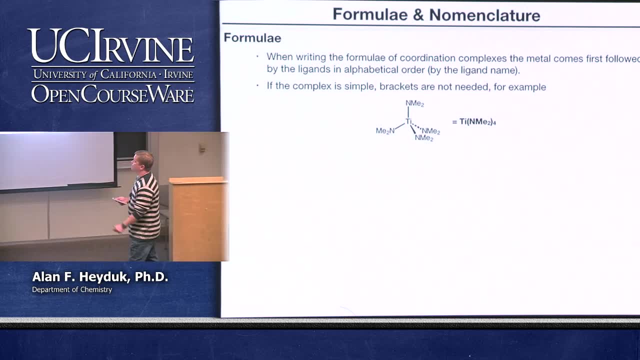 you know what I'm talking about. All right, So we'll start by writing formulas. When you write the formula of a transition metal compound, the metal comes first because it's the most important. We typically go with the ligands in alphabetical order by the ligand name, not by the formula of the ligand. 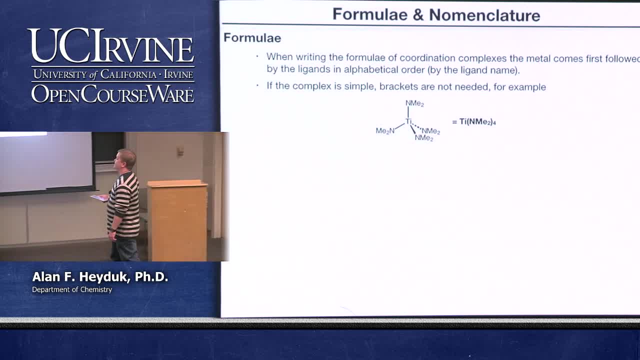 And so if the complex is simple, brackets are not needed. For example, this tetrakis dimethylamide titanium complex. Well, there, that should confuse you, because you'll notice that when I gave you the name, I gave you the ligands first, followed by the metal. 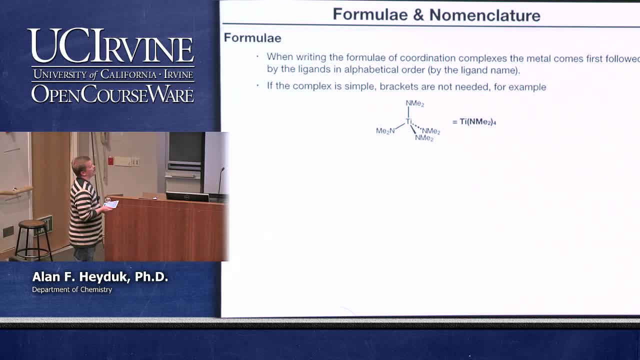 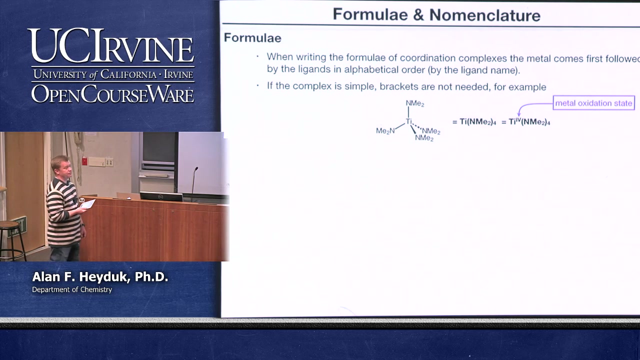 But in the formula we give titanium first And then we just use parentheses to denote the correctly dimethyl azonido or azido ligand, with the four The end. You can also include the oxidation state of the metal in the molecular formula. 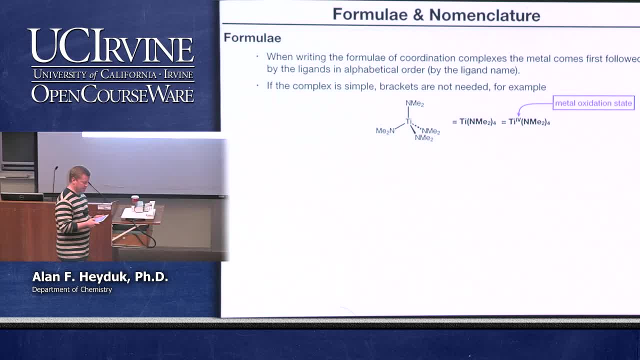 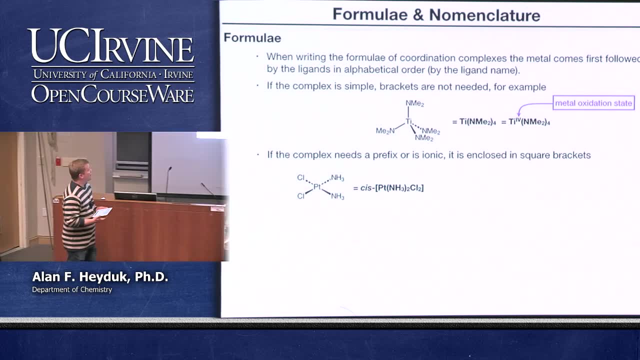 Again, this tells you something about the electronic properties and potential reactivity of the complex, And we'll talk a lot more about this as we go forward. If the complex needs a prefix or is ionic, we use square brackets. So here's our cancer drug, cisplatin. 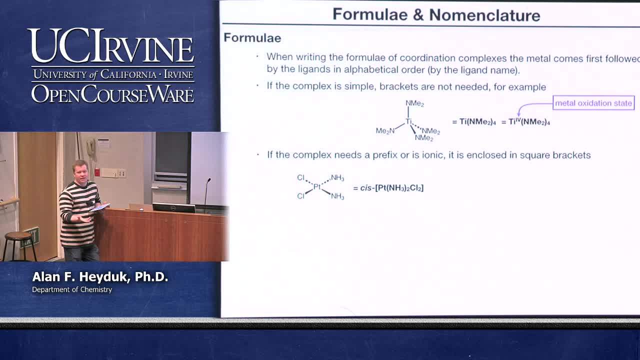 So, just like with an organic compound, we use square brackets. Just like with an organic compound, you have to give the regiochemistry, You have to give that cis in order to tell everybody that the chlorides are related to each other by 90 degrees. 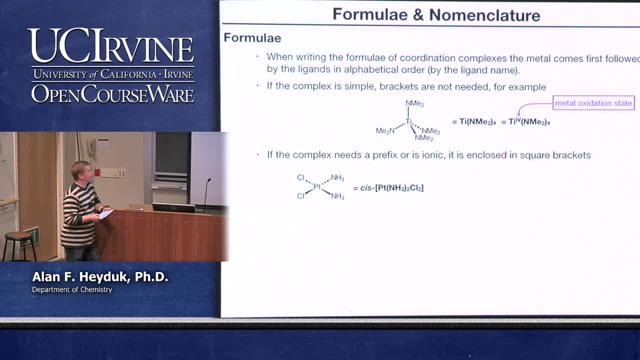 and the ammonia malt ligands are related to each other by 90 degrees. You only need one cis, because a schooled inorganic chemist will know that this compound has to be square planar And if the chlorides are cis to one another, 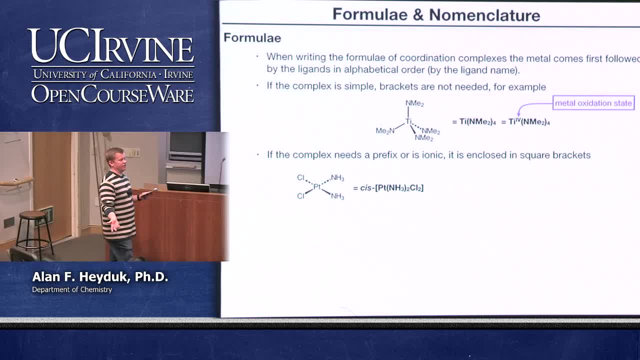 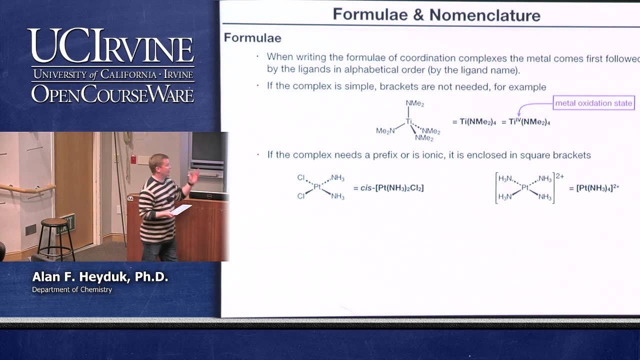 then by definition, the only two spots left to the ammonia ligands are cis to one another. So you don't need cis, cis, platinum diammonia dichloride, You just need the one cis- Same thing. So another example now for a dicat ion. 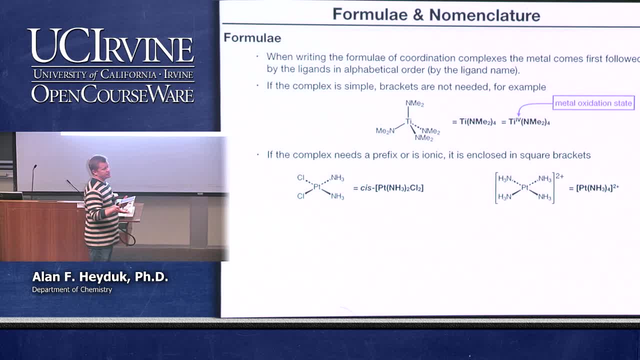 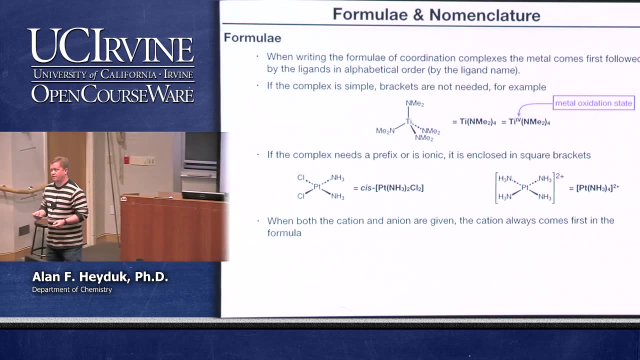 The platinum with four ammonias would go in square brackets with either the two plus, if you're just talking about the cation, or you could have the counter anions listed after it, also in square brackets, to denote the total formulation of the salt. 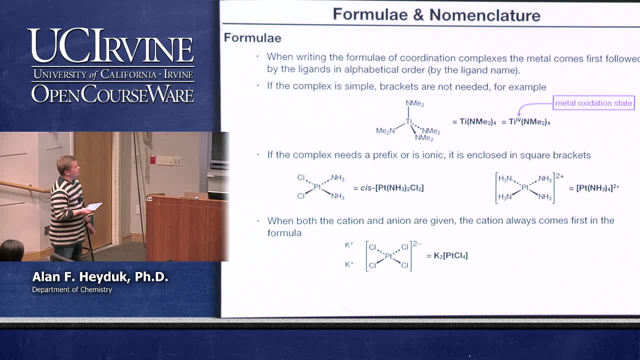 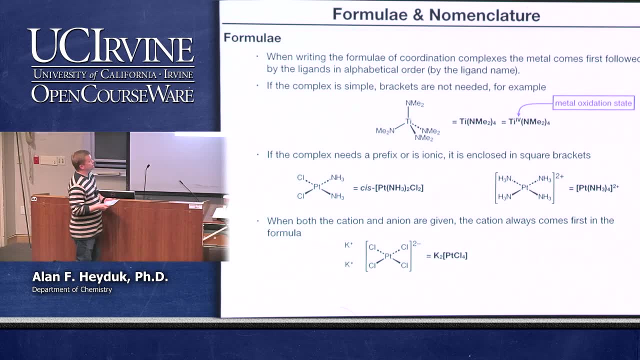 So here's an example: The dipotassium tetrachloroplatinate. The cations come first. So two potassium. The potassiums can be in brackets. They don't have to be in brackets So often they're left out. 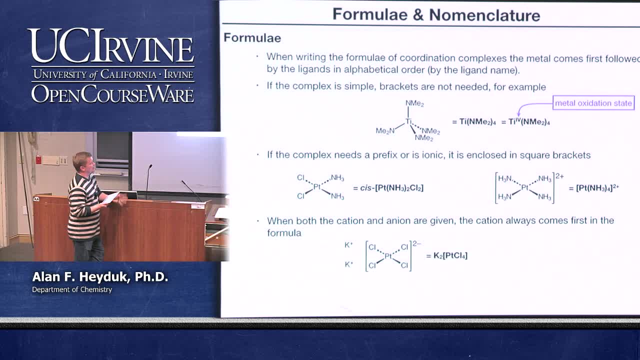 The tetrachloroplatinate goes in brackets because it's an anion and it comes second. If we include the oxidation state, it goes inside the brackets as a superscript following the platinum element. We never give the oxidation state for the ligands. 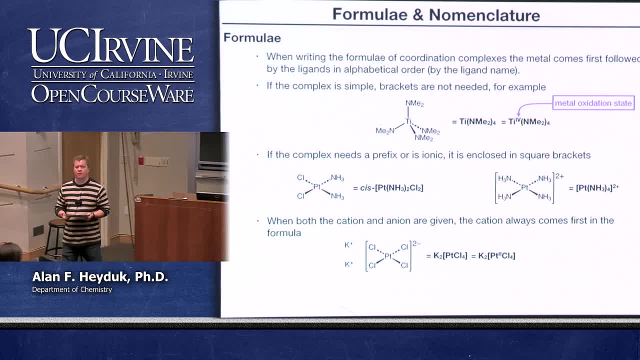 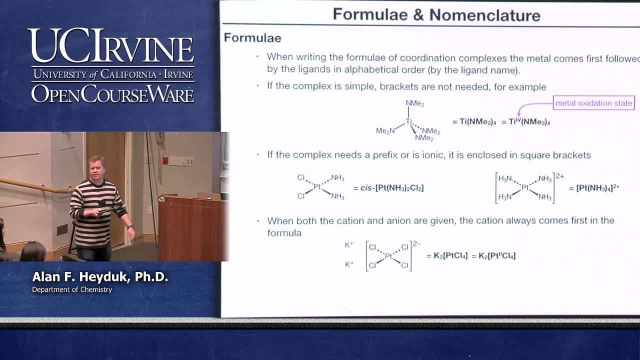 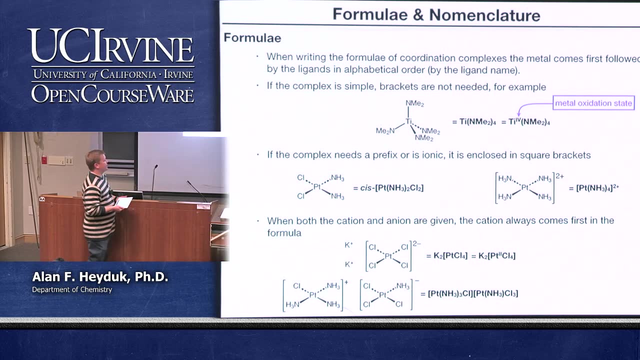 okay with. there are some exceptions, but we won't get to those in this class Because, frankly, the ligands are just, you know, there to support the metal, which is the cool part, And here's an example where we have both the cation and the anion fully spelled out. 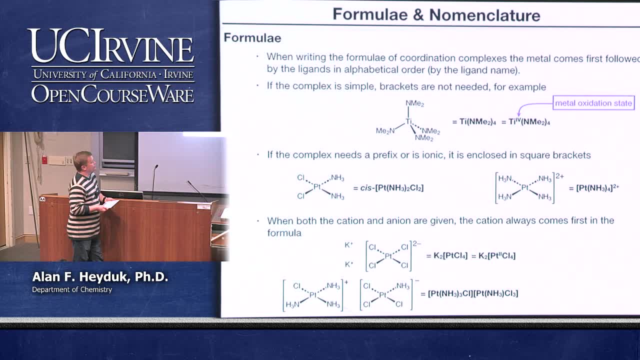 Both of them are the charged platinum complexes. You'll notice within each set of square brackets, the platinum comes first, followed by the ammonia ligand, because ammonia starts with A and it is first letter in the alphabet. And then last is the chloride, because C comes after A. 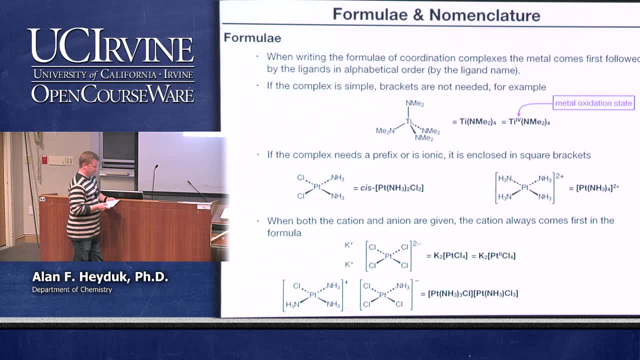 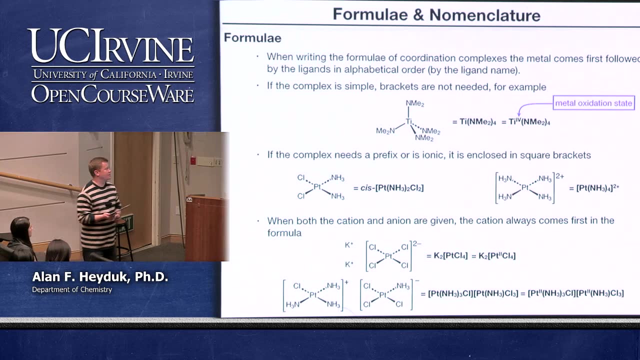 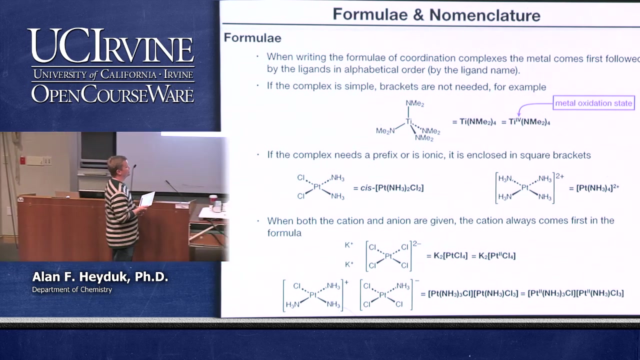 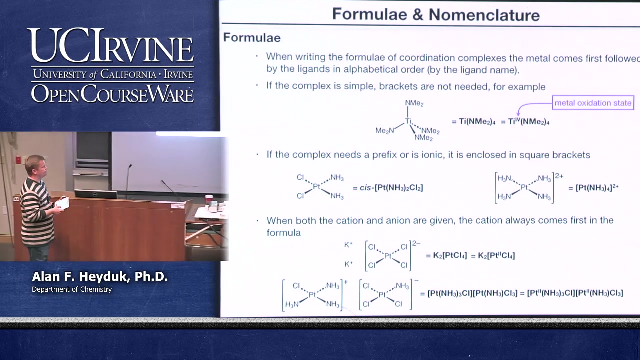 And we do things alphabetically for the formulas Again, for this combination of the platinum, the platinum dication and the die or sorry mono cation and mono anion. Both platinum centers are in the plus two oxidation state, but we would indicate them individually if we chose to include the oxidation state in the formula. 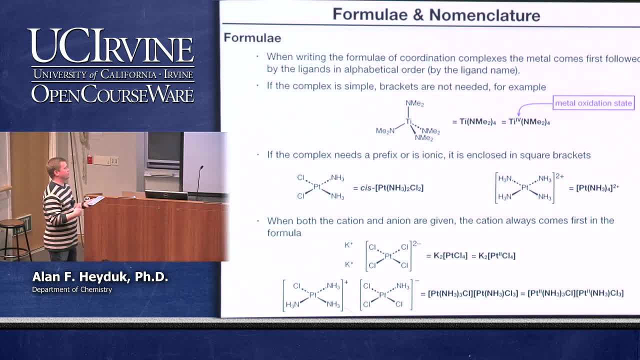 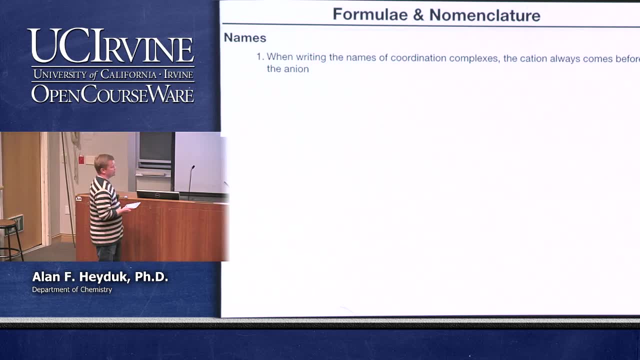 Not required but often helps you or the reader or whoever, keep track of what the oxidation state is. Okay, so let's talk about formulas. Formulas are pretty easy. The names are a little bit more complicated. So first rule, when you write the name of a coordination complex, 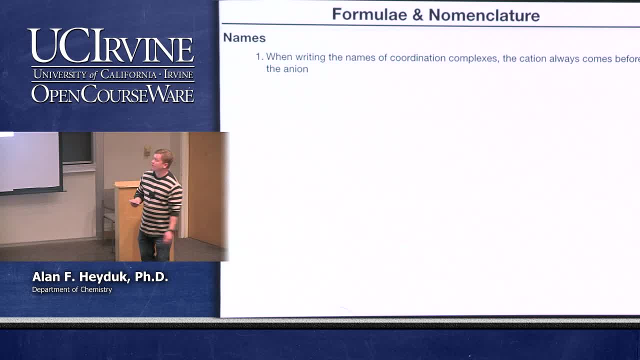 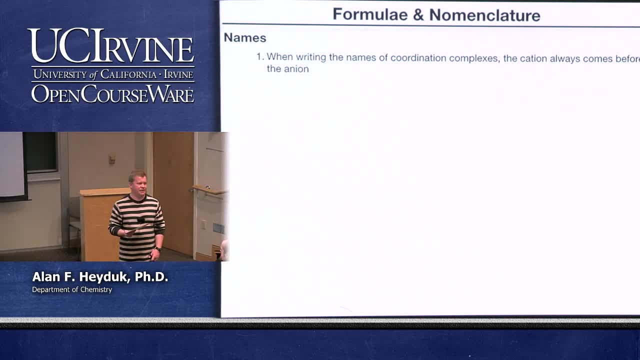 the name of the cation always becomes before the name of the anion. Okay, we never talk about chloride sodium. I mean you guys know this right. It's kind of a silly rule: Cation always comes first. The ligands are listed alphabetically: 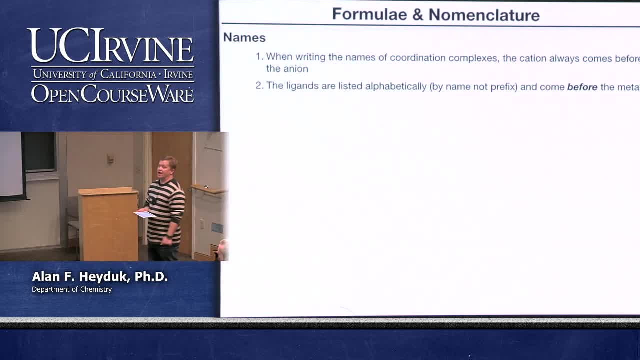 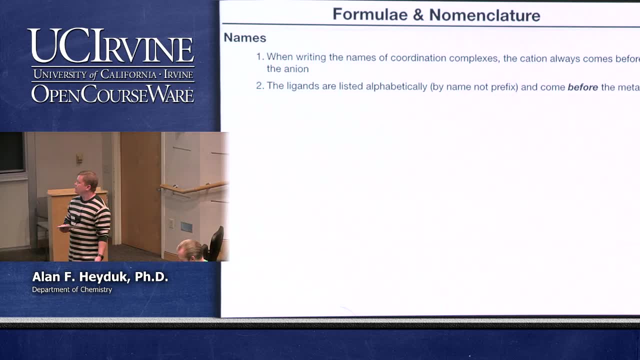 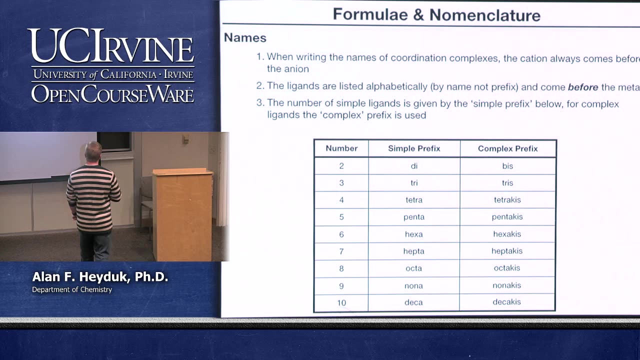 Name, not prefix. So if you have an ammonia ligand, it goes by A. If you have four ammonia ligands, it doesn't go by tetra, it goes by A. The number of simple ligands is given by a simple prefix. 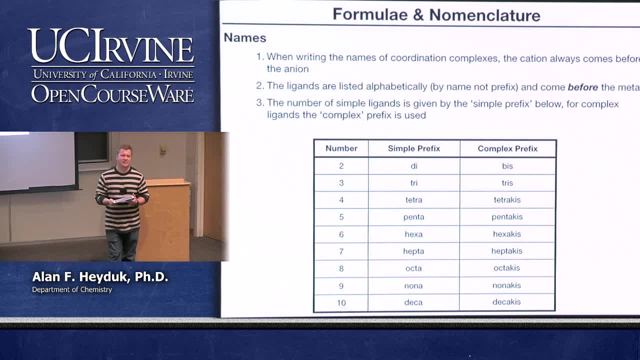 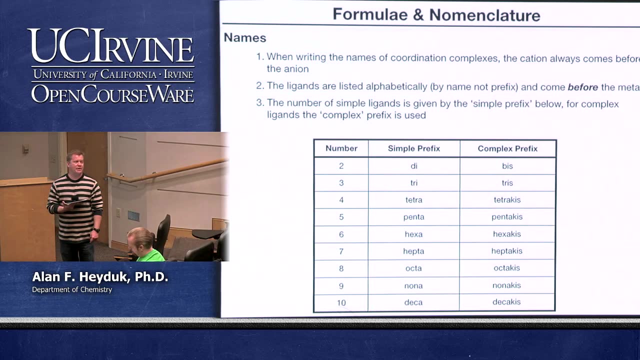 For complex ligands, the complex prefix is used. This is where you should just roll your eyes and go. are you kidding me? Okay, why in the world would you have simple prefixes and complex prefixes? I mean, it wouldn't be too confusing to have three triethylamines bound to a metal. 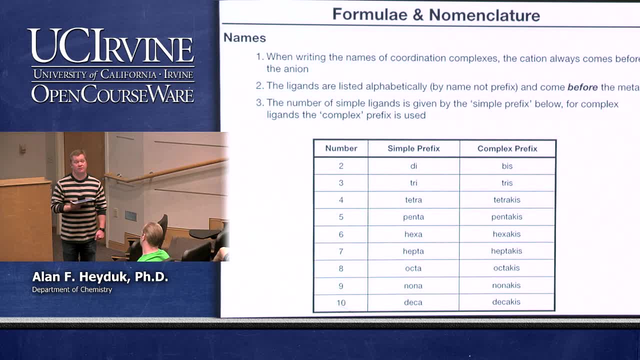 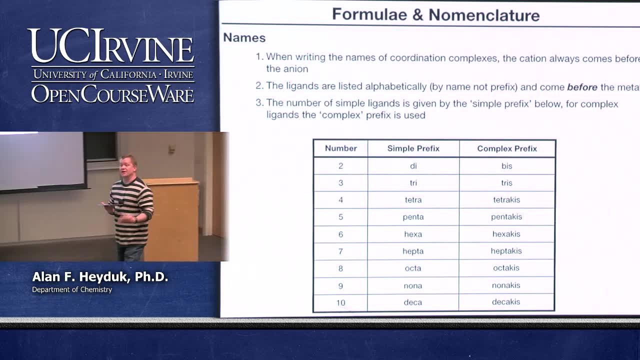 right. If we use the simple prefix, it would be tri-triethylamine, Like you know, tri-tri-harder or something. So no, that would be a tris-triethylamine. So that's literally why we have simple prefixes and complex prefixes. 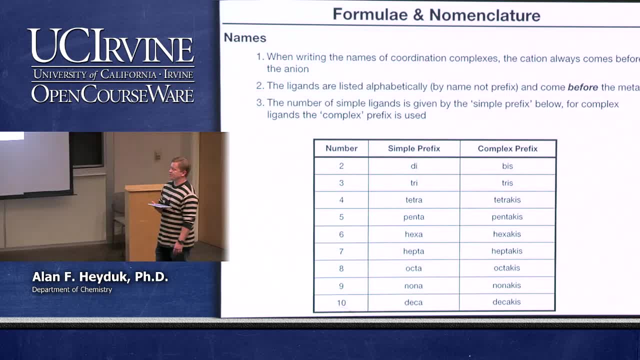 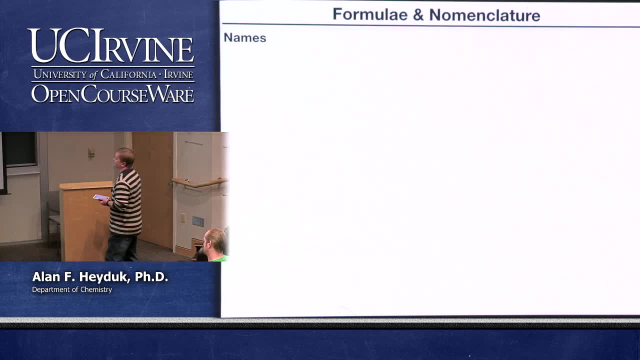 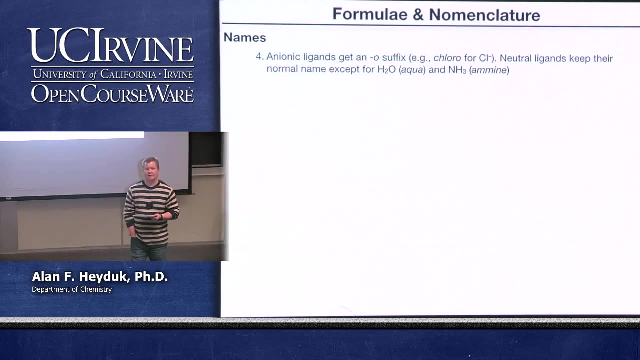 Because it just starts to sound ridiculous. if you know you have three tries in a row. Number four, Anionic ligands, get an O suffix. So every time you hear me say chloride up here, you should scoff at me and say: 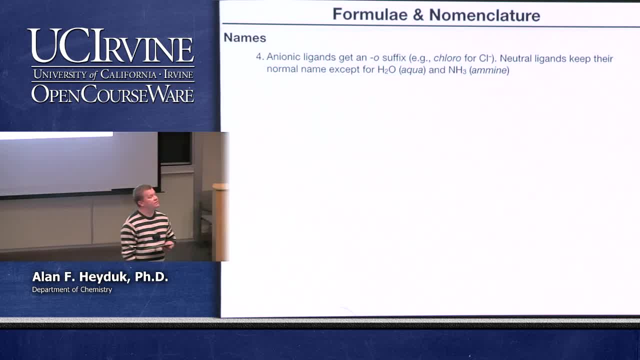 you're wrong. It's not a chloride ligand. it's a chloro-ligand, because it's an anionic ligand and it gets an O suffix. Neutral ligands keep their normal names, except for a few isolated examples where we have to trick you and have special names. 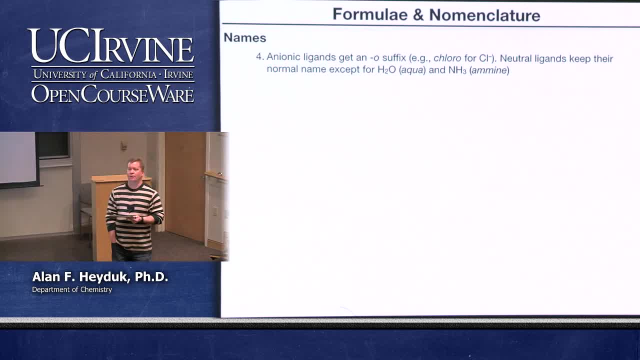 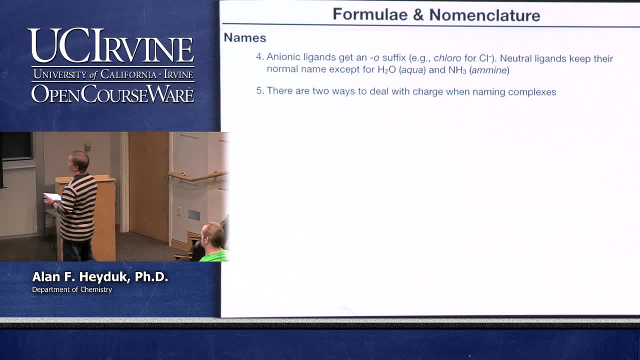 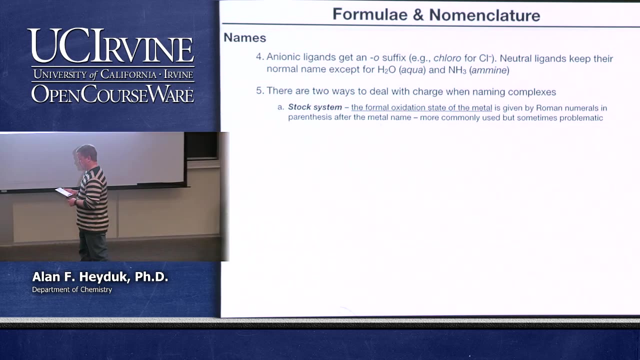 So it's not a water ligand, it's an aqua ligand. it's not an ammonia ligand, it's an amine ligand. There are two ways to deal with charge when you name a complex. The first is in the stock system. 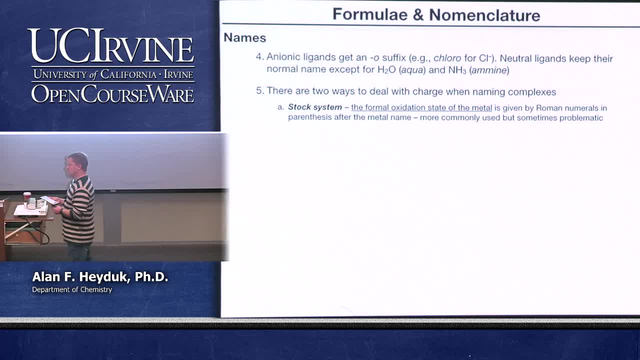 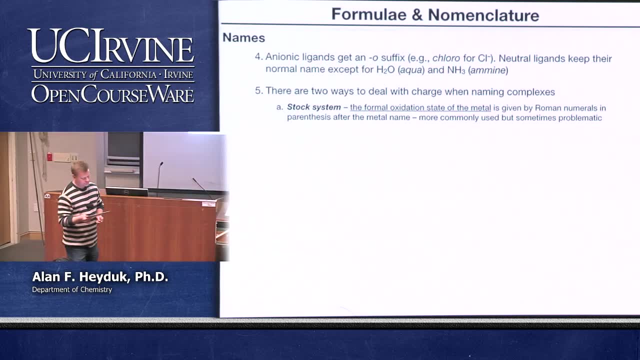 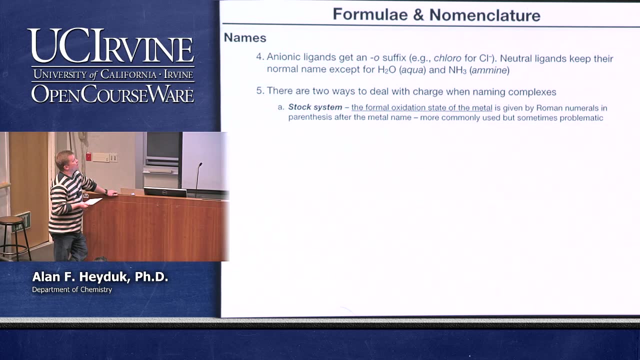 And in that case you give the formal oxidation state of the metal and it's given by a Roman numeral in parentheses after the name of the complex or specifically the metal. This is commonly used but it can be problematic. We'll see some of the problems that come up. 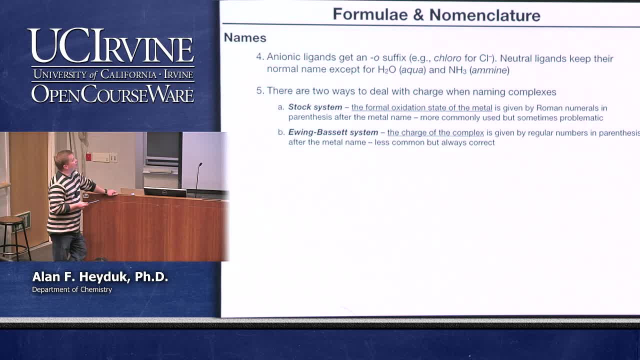 The other is the Ewing-Bassett system. In the Ewing-Bassett system you give the charge of the complex And in the Ewing-Bassett system you give the charge of the complex. It's given by a regular number. 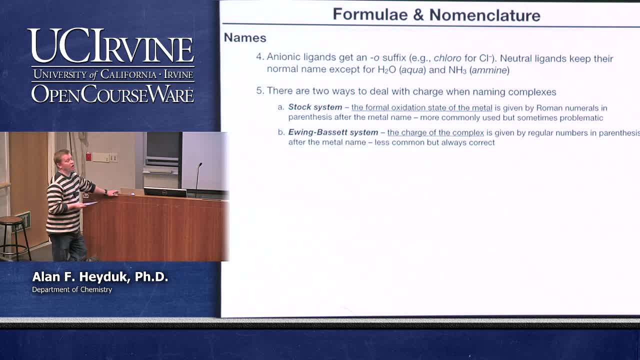 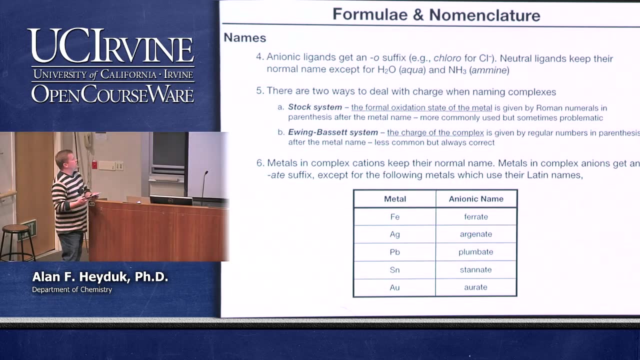 in parentheses after the metal name. It's less common, but it's always correct. We will see examples, so we're going to go through a whole ton of examples on the next couple of slides. So metals and complex cations keep their normal name. 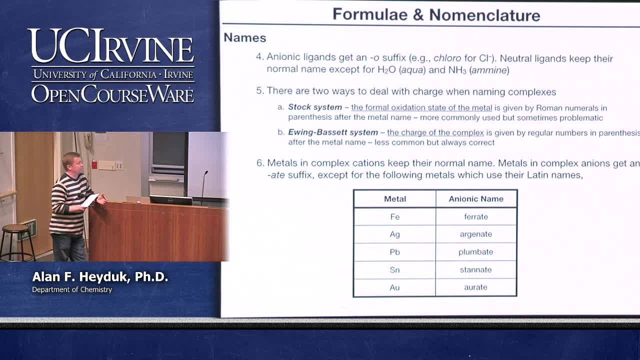 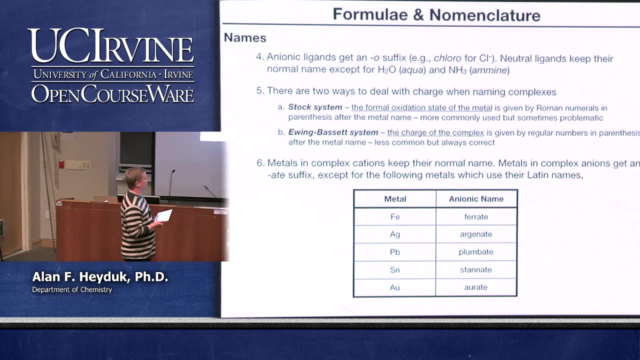 Metals and complex anions get an 8, so platinate, for example, except for the oddball metals that you always wondered why they have that symbol on the periodic table. So if you have an anion for iron, it's ferrate. 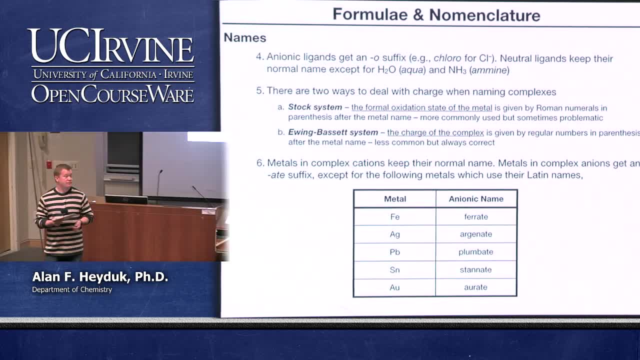 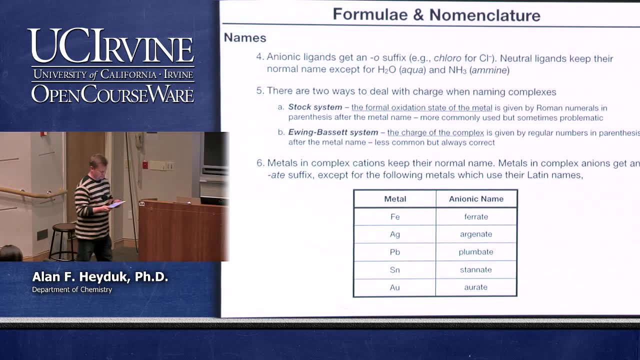 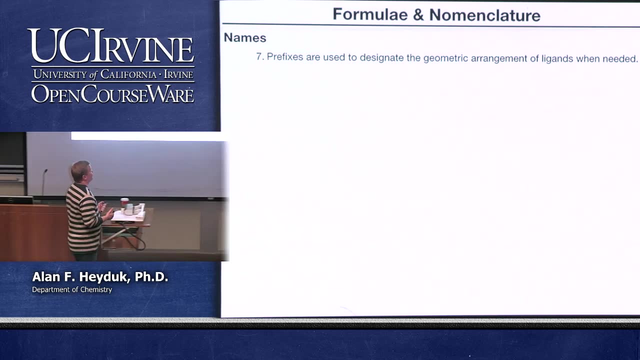 If you have an anion of a silver complex, it's arginate. Plumbate, because you know that's what plumbers do: Stanate, orate, so on and so forth. Okay, Prefixes are used to designate. 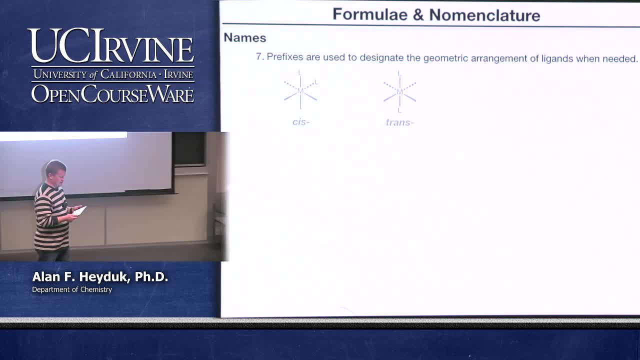 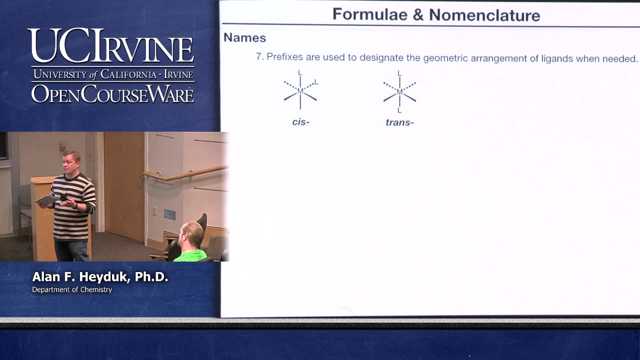 the geometric arrangement of ligands when needed. We've seen cis and trans already. Cis and trans come up in square planar geometries. They come up in octahedral geometries. They can come up in trigonal bipyramidal geometries. 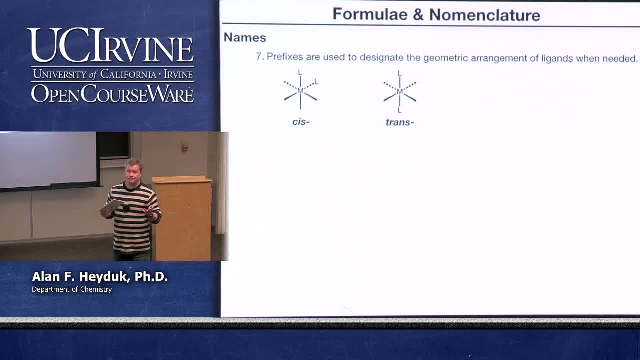 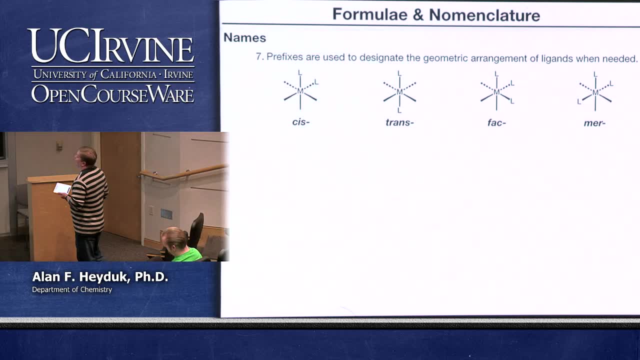 You never have to worry about cis and trans. if you have a tetrahedron, Okay, Because all of the angles are equal. A special one for octahedral complexes is fac and mer: Fac for facial, mer for meridional. 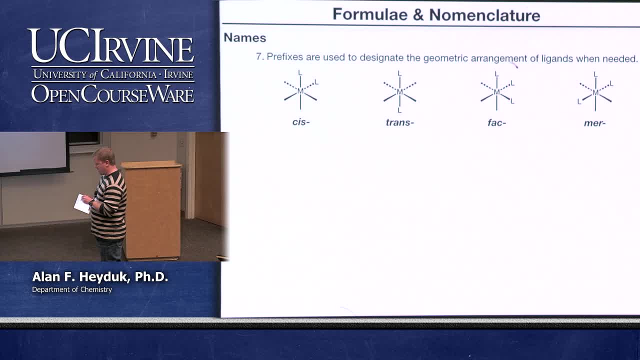 Okay, In the facial arrangement you have three ligands on a single trigonal face of the octahedron. For the mer arrangement, instead, you have three ligands on the meridian. I think of it as being a belt around the metal complex. 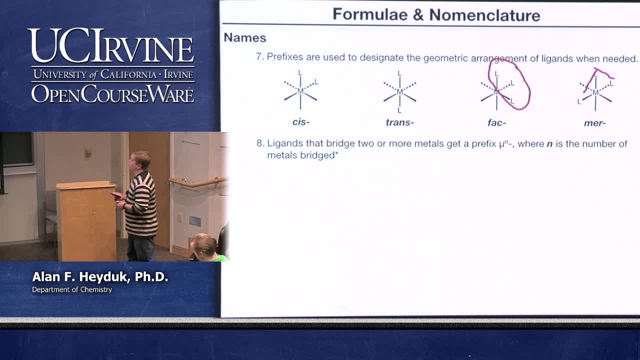 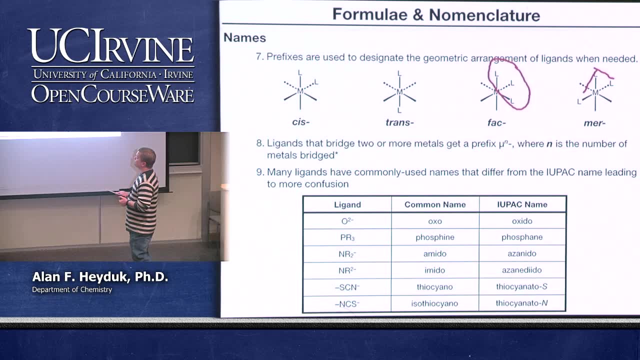 Ligands that bridge two or more metals get a prefix mu with a superscript n. n is the number of metals bridged. We've seen this for. We saw that for sulfur. Thanks for the reminder. I have office hours in 15 minutes. 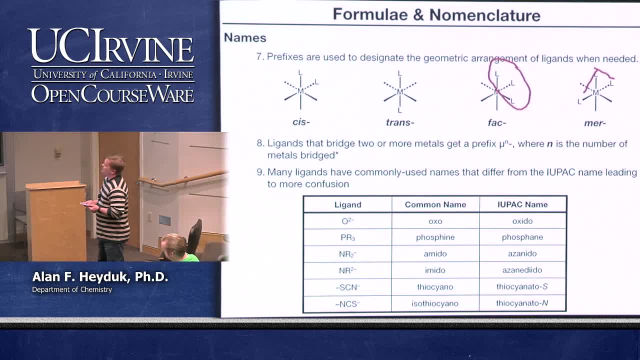 And then we have Many ligands have commonly used names that differ from IUPAC name, leading to even more confusion. So we've all seen this. for organic chemistry It's worse for inorganic chemistry And just like organic chemists who you know, 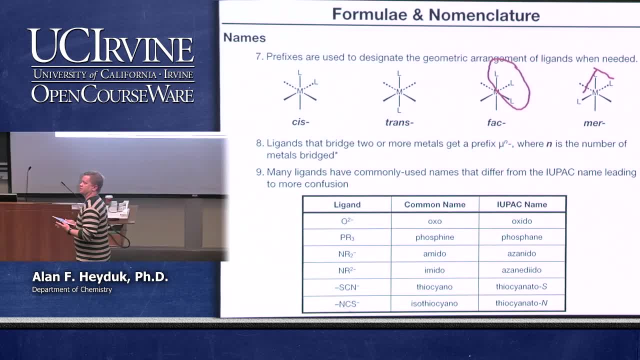 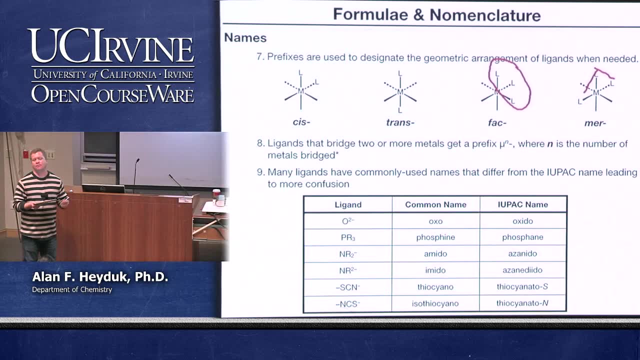 refuse to refer to use IUPAC names and they use the trivial or common names. inorganic chemists do the same thing. I can almost promise you, outside of this classroom, I will never talk to you about a metal-oxido complex. 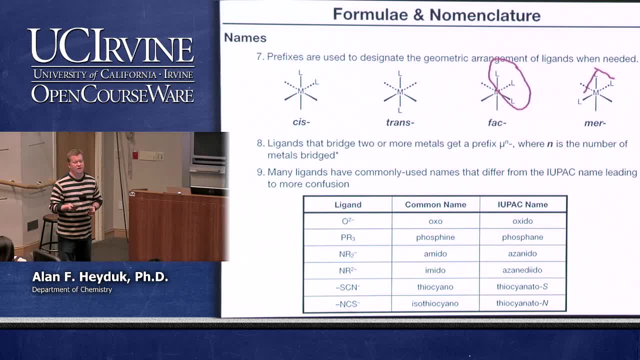 which would be the appropriate name for a metal complex with an O2 minus a metal-oxygen double bond. I guarantee I will always refer to it as a metal-oxygen double bond. Okay, Inside of this classroom it's 50-50.. 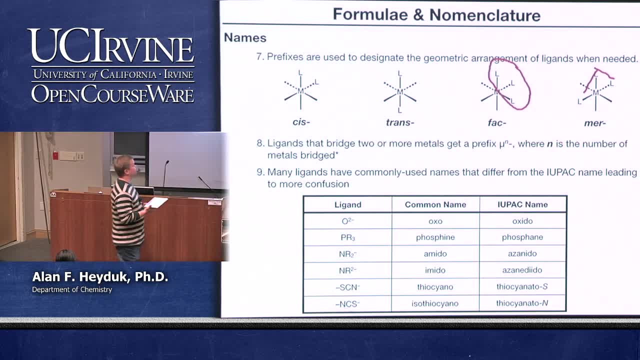 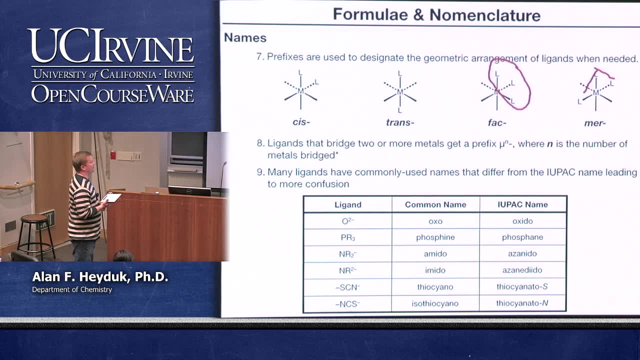 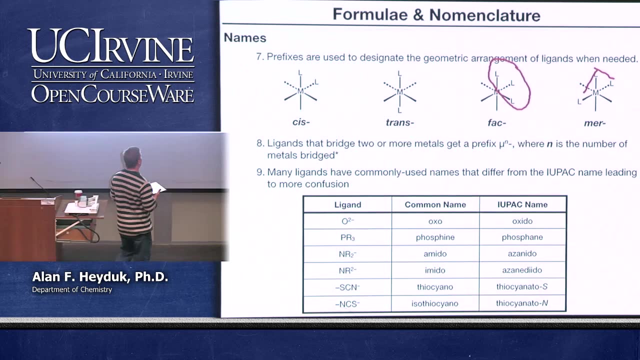 We'll see. PR3 will exclusively be referred to as phosphenes, but they're phosphenes, NR2 minus inorganic chemists always refer to these as amido ligands. Okay, And then they'll get lazy. 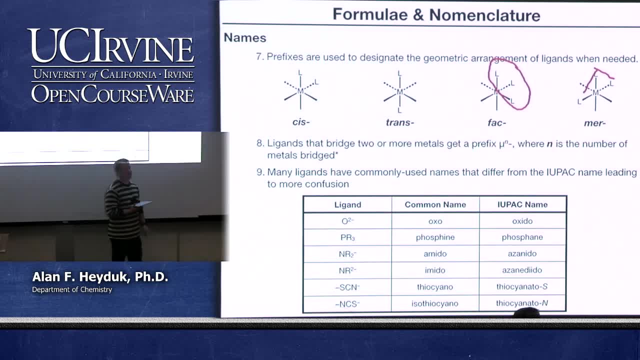 and they'll talk about amides, And every organic chemist goes: amido ligands, Amido ligands. Where's the carbonyl oxygen? Right, Because that's what an amide is. And so this is where you see. 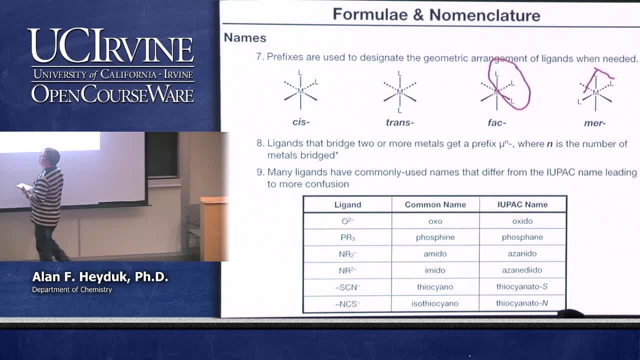 how you name things becomes important, And so we should really be calling that an azonido. And so there's a whole list in your book of the proper IUPAC name for a bunch of different functional groups or ligands in transition metals. 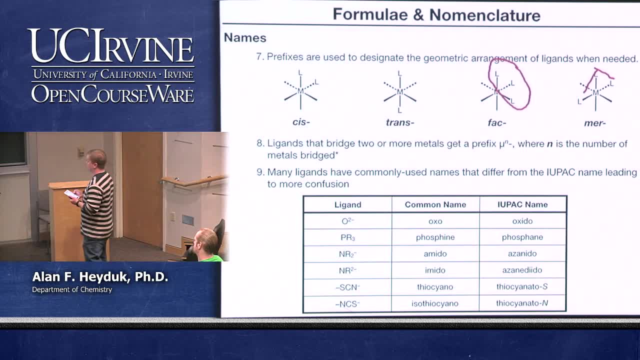 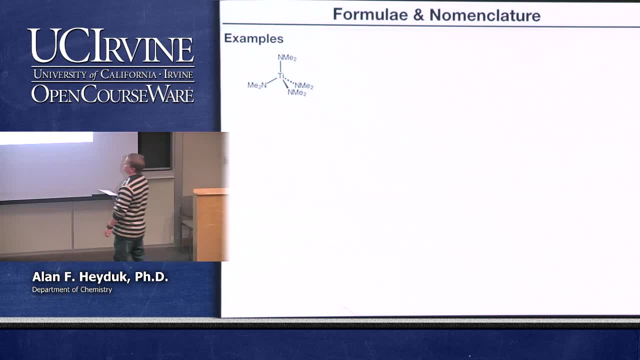 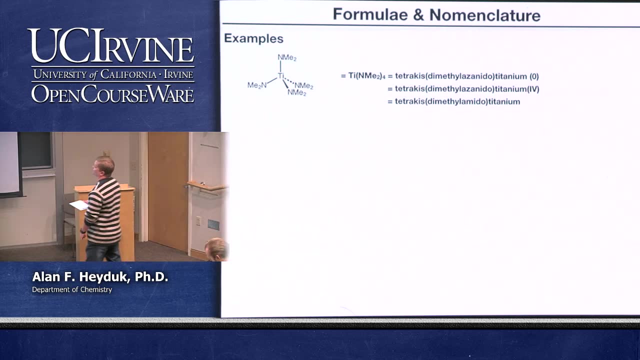 And we do need to make a real effort to be consistent. Okay, We'll very quickly go through a couple of examples before we break for the day. So we've seen this. We know how to write the formula: The titanium comes first. 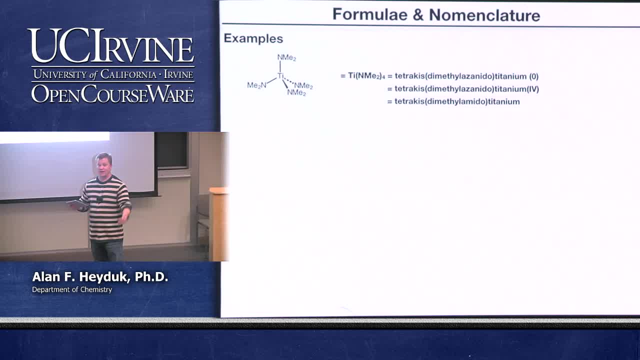 Then we put the dimethyl azonido ligand in parentheses with the subscript for, But when we come to name it we flip and the ligand comes first. So tetrakis dimethyl azonido titanium, So the first thing. 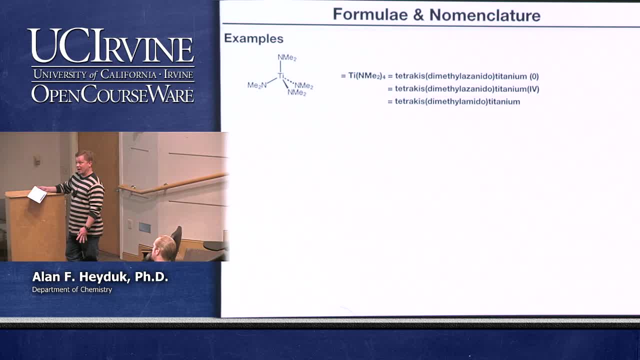 the first example that I've given. I have a regular- I guess it's a Latin digit- in parentheses with a space after the name. So that's the Ewing-Bassett formalism to indicate charge And it's telling you that the charge. 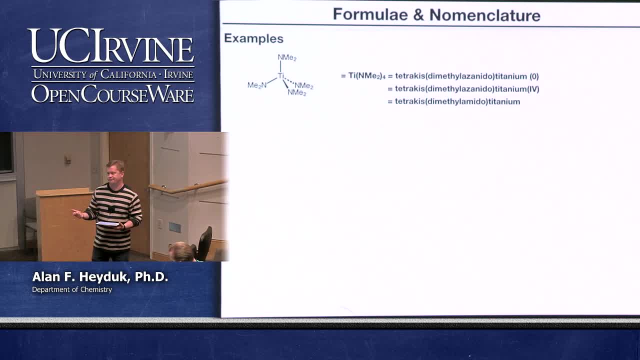 on the metal complex is zero. Okay, It's absolutely correct. The second one that I've put up there: tetrakis dimethyl azonido titanium, no space parentheses. Roman numeral four: This is the stock system for charge. 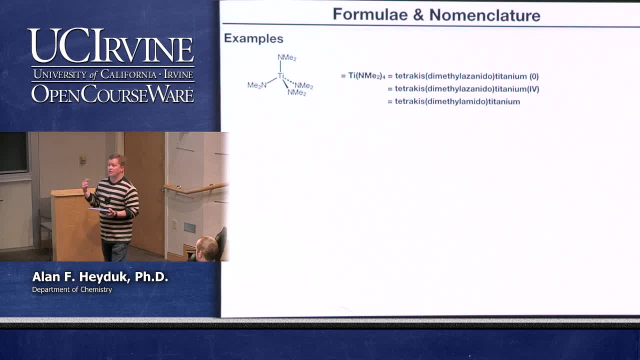 Now it's four, because the stock system gives you the oxidation state of the transition metal. Sometimes that can be problematic. Now how do you reconcile The Ewing-Bassett system saying that the charge on the complex is zero with the stock system saying 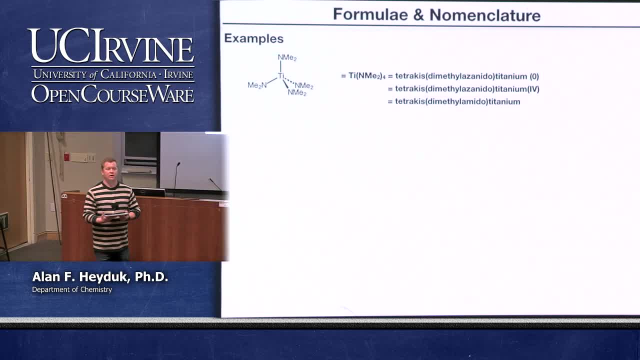 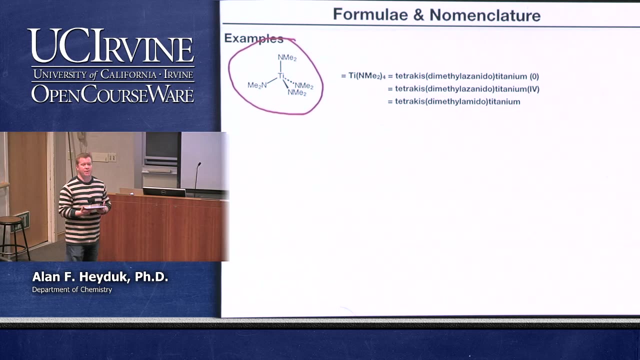 that the oxidation state is four. Well, they're in a way referring to different things. Okay, We know to assign the oxidation state to this metal or to the metal to the titanium center. in this complex, we take each pair of electrons. 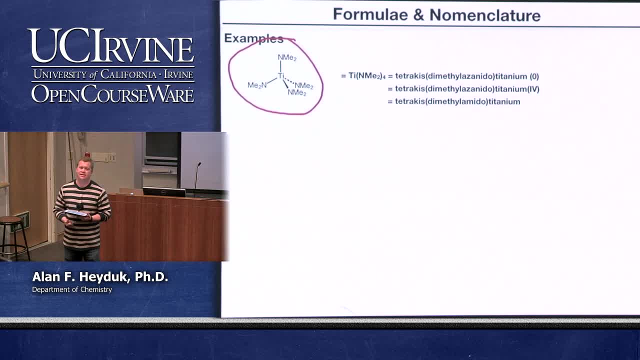 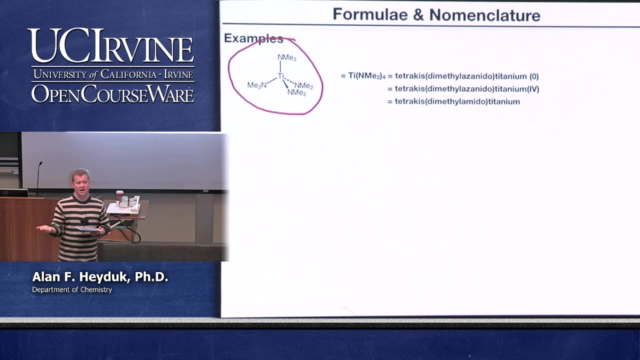 that make a metal-ligand-sigma bond and assign them to the more electronegative element. Nitrogen is more electronegative than titanium, So the electrons in that sigma bond get assigned to the dimethyl azonido ligand. 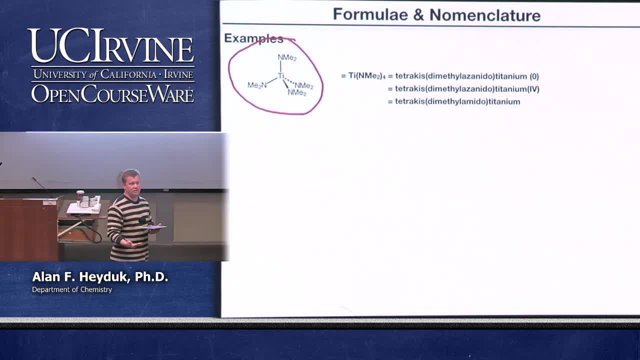 So each one of those ligands is a minus one ligand. That means we've basically taken all of titanium's electrons from it, and so it has an oxidation state of plus four: A titanium with a plus four charge and four mono-anionic ligands.